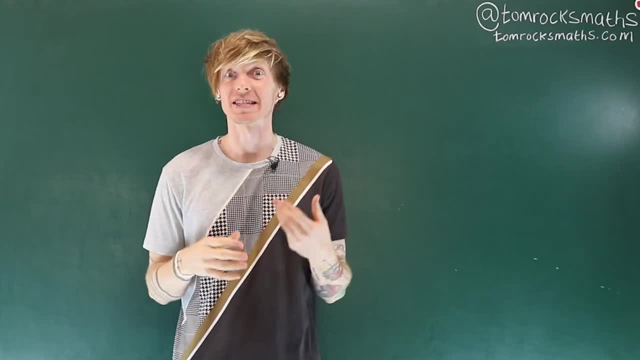 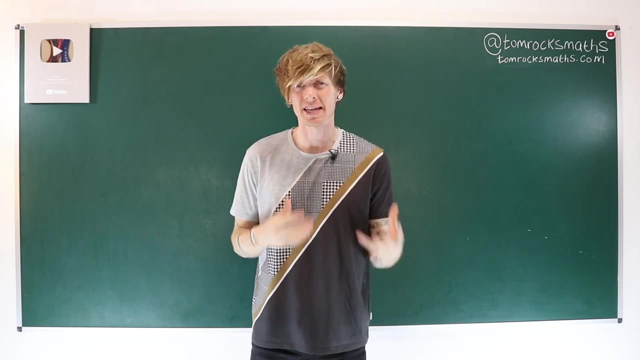 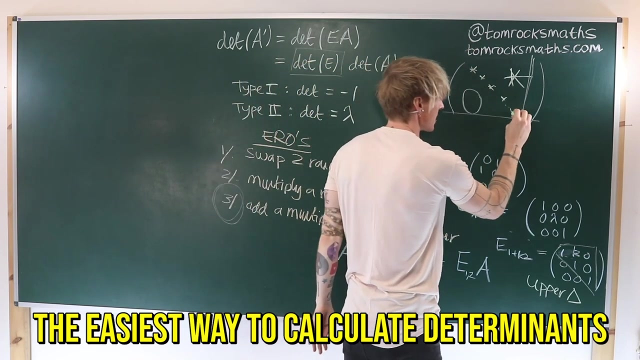 Hello math fans, Dr Tom Crawford, here at the University of Oxford, and today we're looking at the vector space axioms. So far in the Oxford Linear Algebra series, we've been mainly focusing on matrices and their associated properties, such as determinants, eigenvalues and eigenvectors. 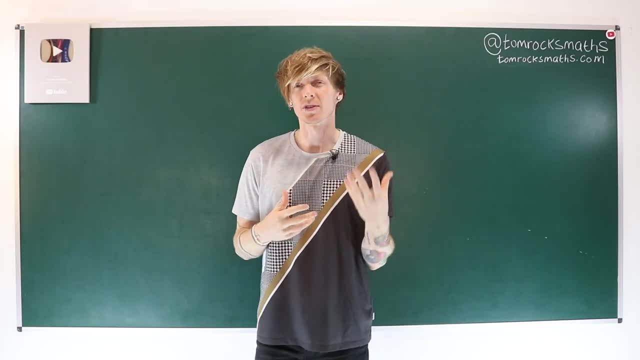 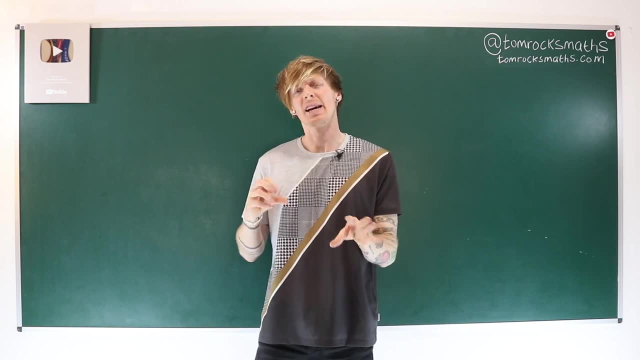 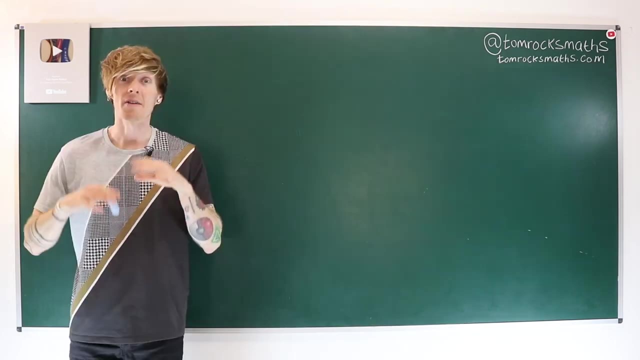 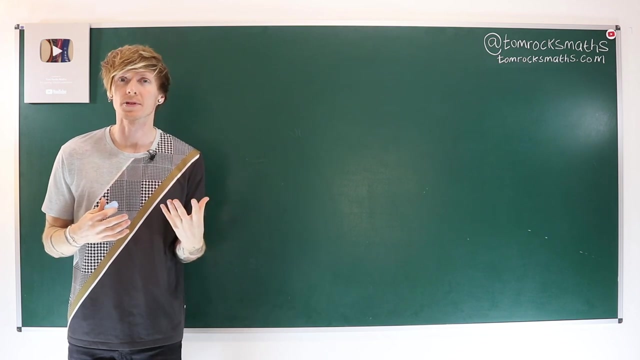 But to really understand the usefulness and universality of matrices, we actually need to take a step back and look at things in a more abstract setting, And this is where vector spaces come in. A vector space is a mathematical object which satisfies a series of rules or axioms. 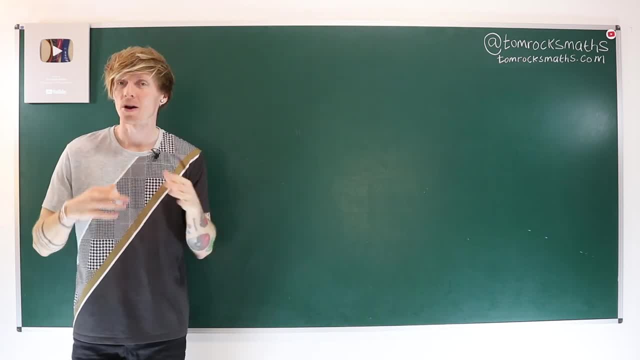 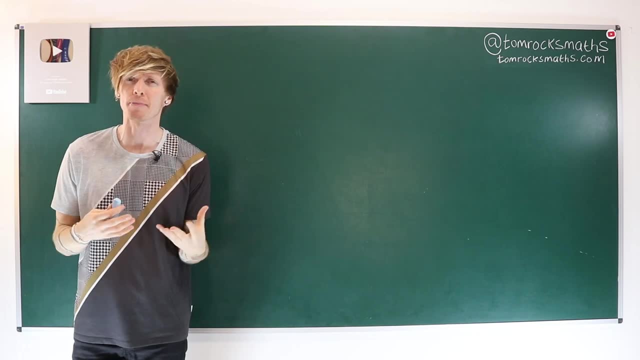 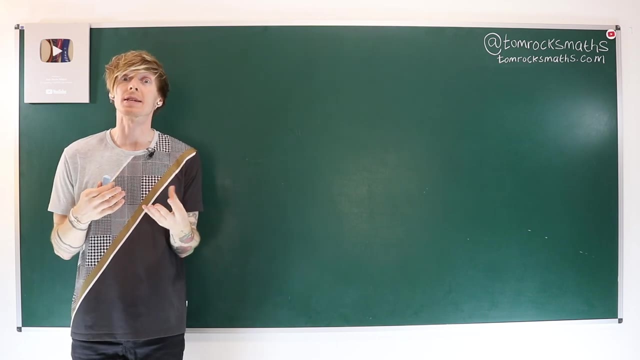 Now I will go through these eight axioms one by one, but I'm going to start with the first one. It's really important that, whilst we do this, you keep in mind the concrete examples with which you are likely familiar. So we have the n? vectors, which simply means a traditional 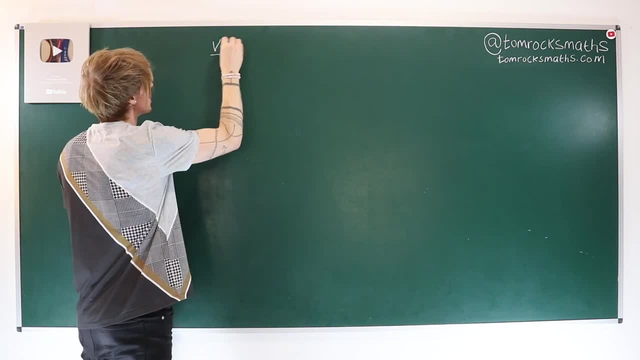 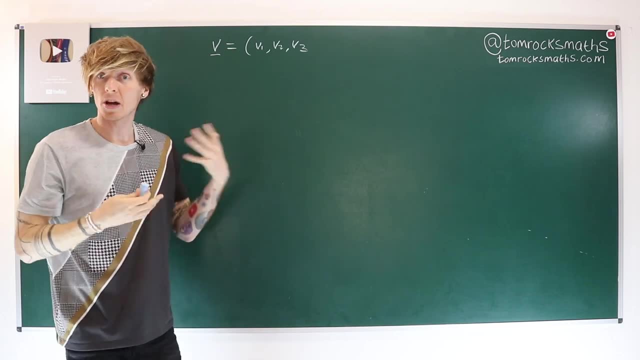 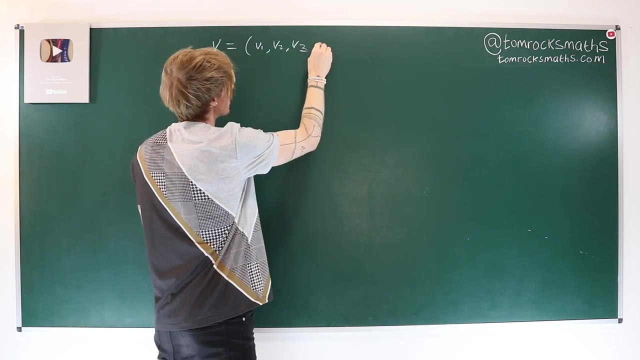 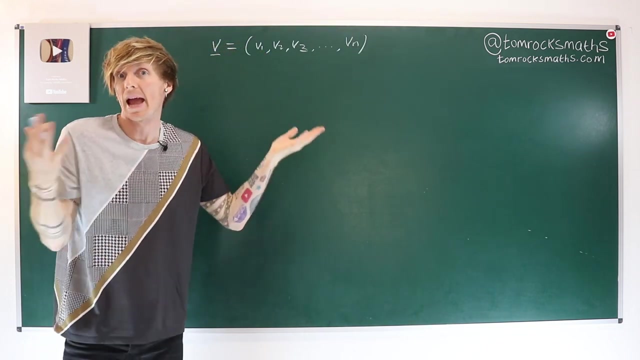 vector. So this could be: v is equal to some entry, v1,, v2,, v3.. And if I were to stop there, that might be a 3d coordinate system. But by an n vector we simply mean there are n coordinates, where n can of course be any number from 1 through to any large integer. 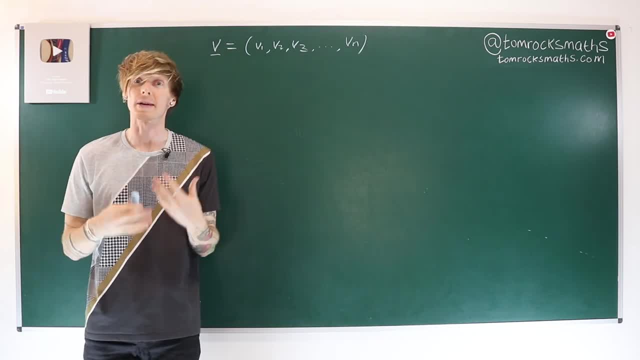 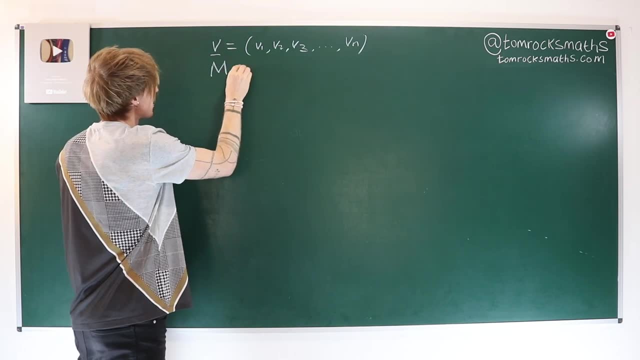 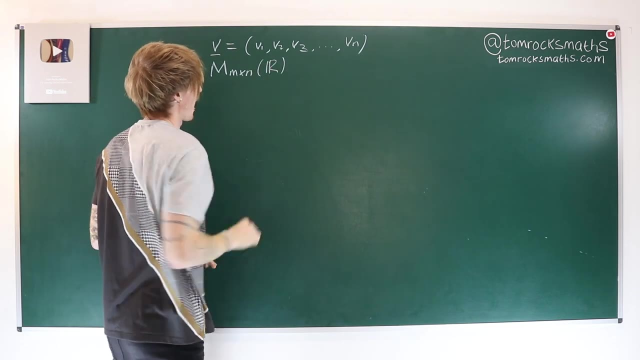 that you can think of. And the second example will of course be matrices, and here I'm going to keep this as general as possible, So we might have the m by n, so they could potentially be rectangular matrices, and let's suppose they have real entries On to the definition. 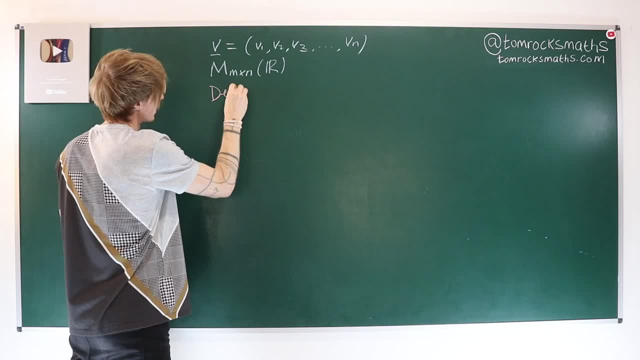 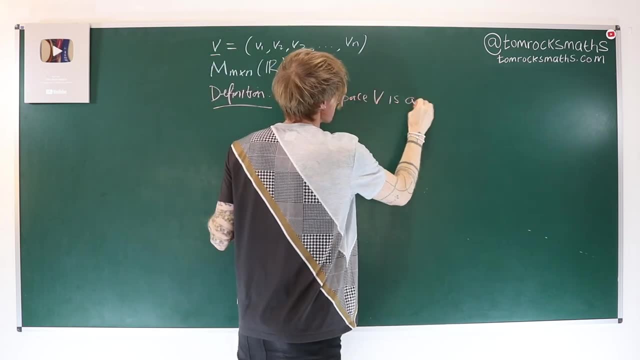 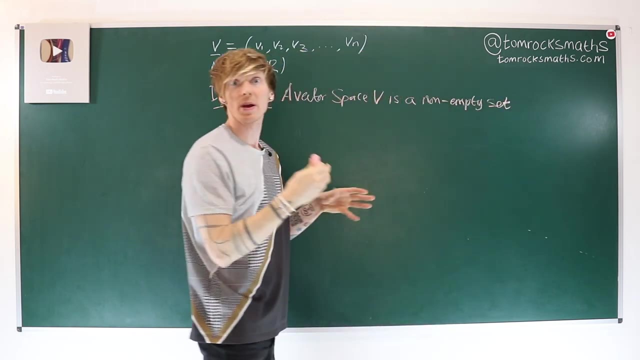 We are going to define the following: A vector space, and let's just label this capital. V is a non-empty set, first and foremost. So we have to have something, some elements on which we are operating on to form this particular structure. So 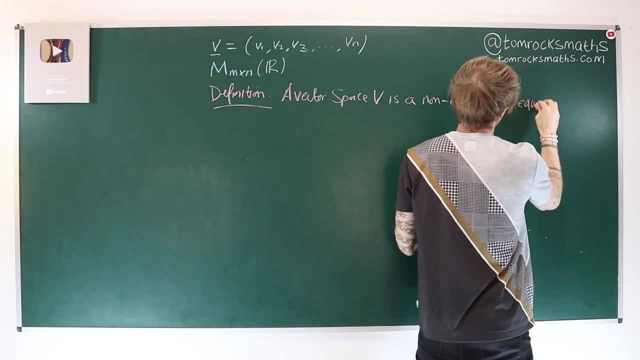 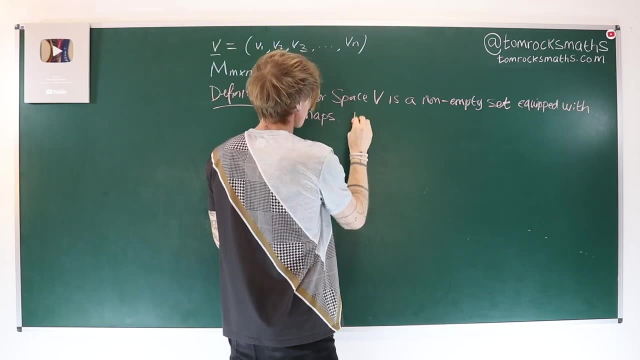 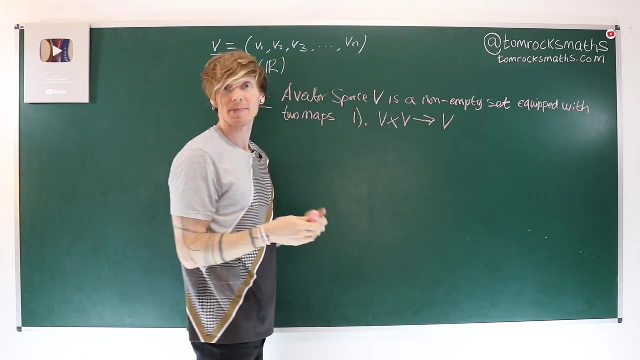 it's going to be a non-empty set equipped with two maps. The first is going to be the addition map, So the addition map is going to be from v, cross v maps into your vector space v, And the way that's going to work is if you input two vectors, u and v. 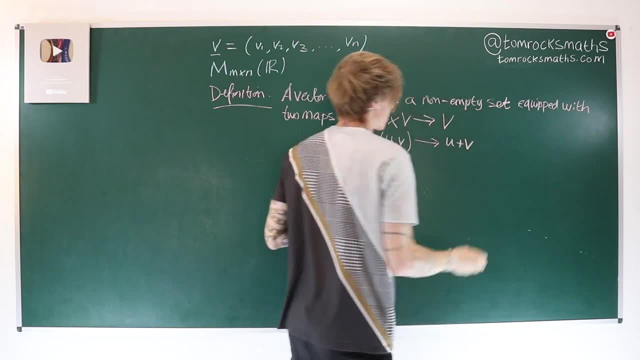 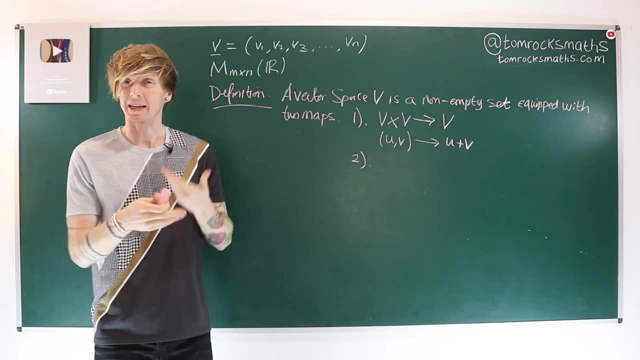 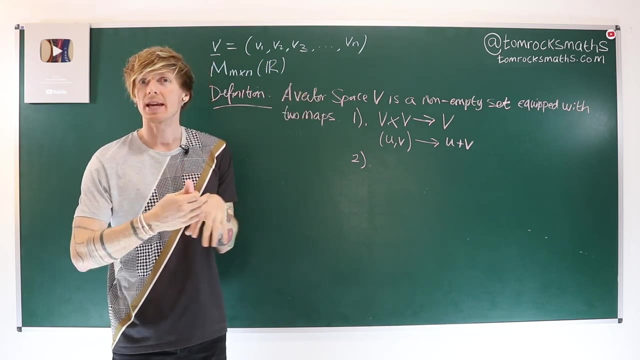 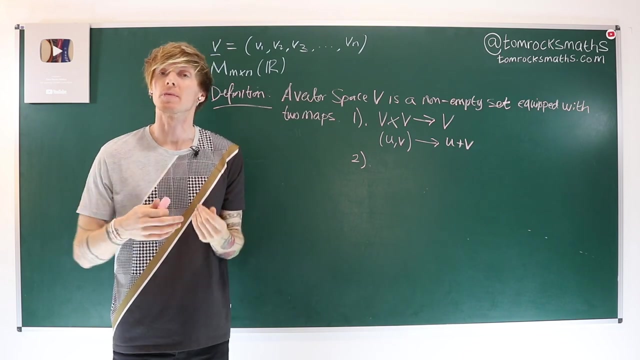 your output is u plus v, as you might expect, And your second map is going to be the scalar multiplication map. And here I'm going to simplify things a little and say: we're going to take our scalar multiples to be in the real numbers. This can in fact be any field, so it could be the complex numbers or other. 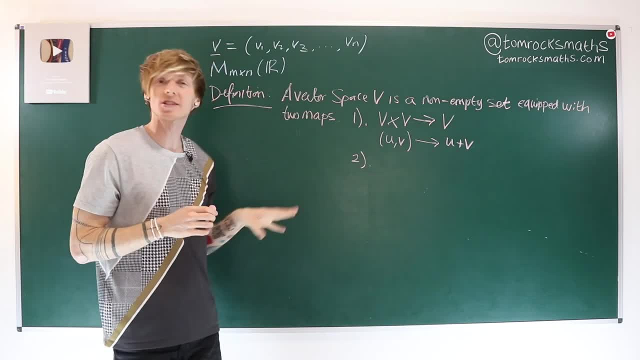 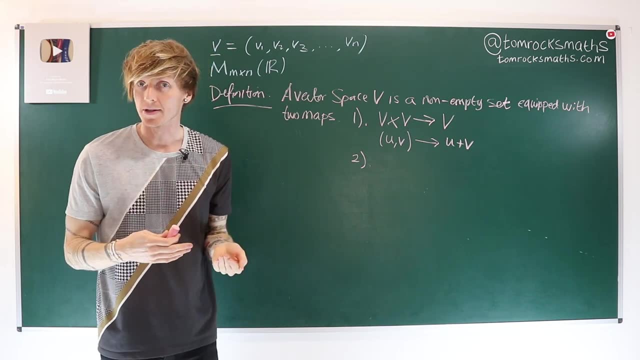 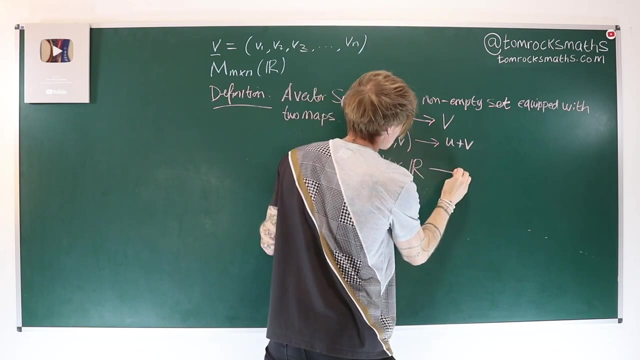 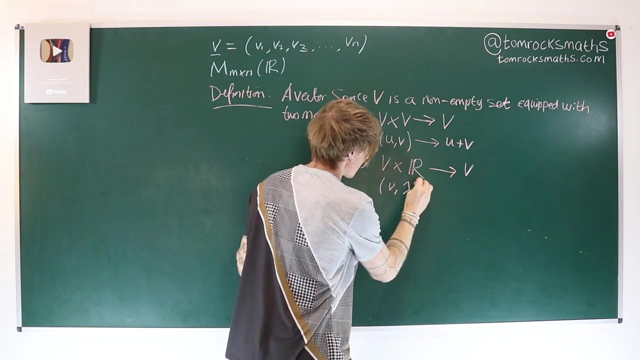 fields which are more advanced. but just to keep things simple here, we will suppose that we are doing scalar multiplication on the real numbers. So this map goes from V, cross the real numbers and that outputs something in V. and the way that one's going to work is we input V and a scalar lambda and that. 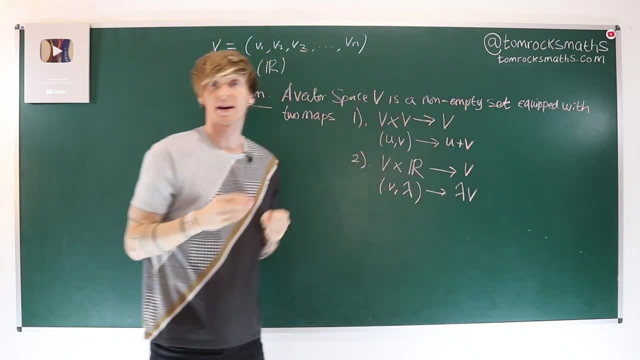 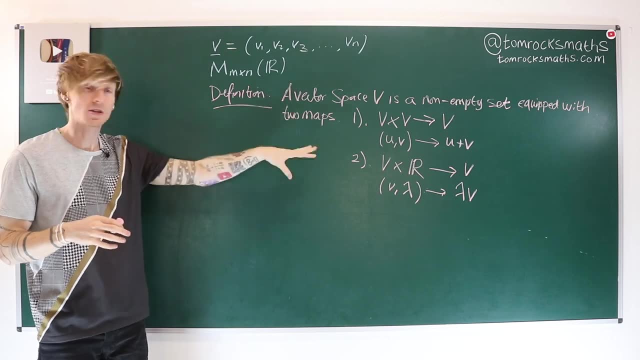 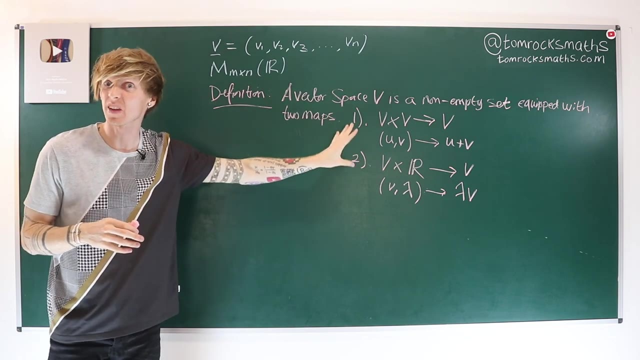 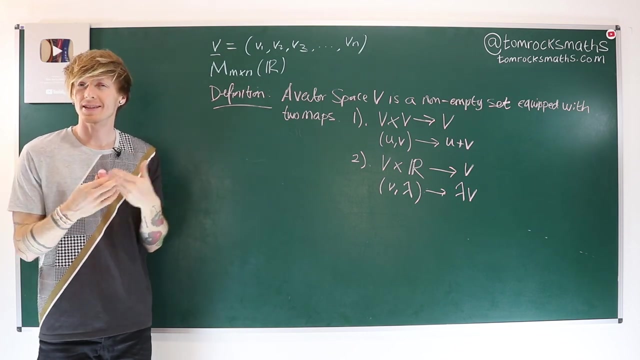 will output lambda times our vector V. So now that we have the setup, with our non-empty set V and our two maps, we have addition or vector addition and subtraction, scalar multiplication with our field, which, remember here we take to be the real numbers. We now need to satisfy the eight vector space axioms. So the first: 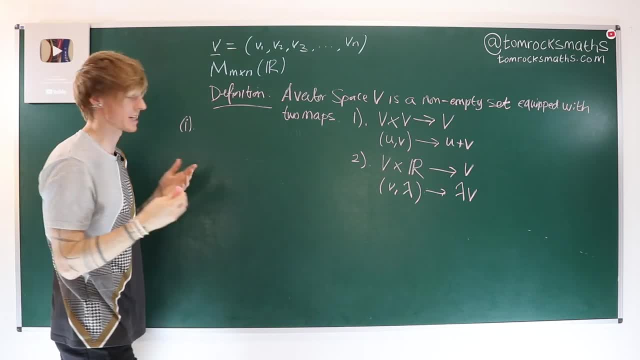 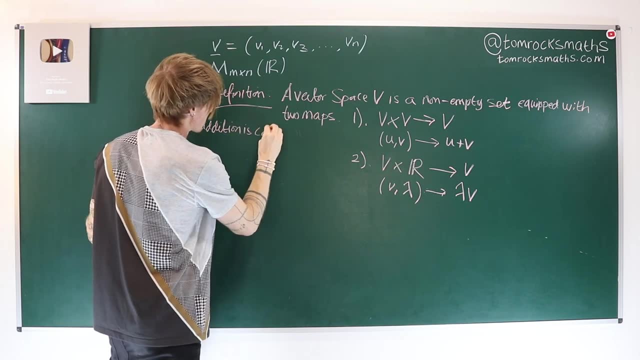 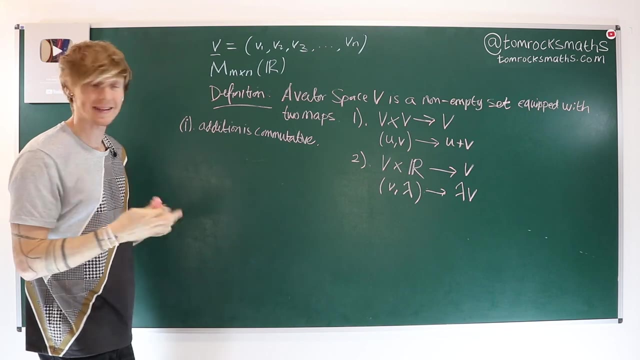 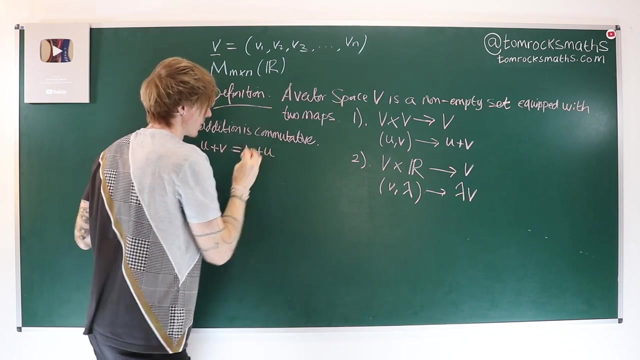 one is that vector addition is going to be commutative, So addition is commutative. Now what this means explicitly is that if I have two vectors, u and v, then that's the same as doing v plus u. Hopefully this is familiar to those of us used to working. 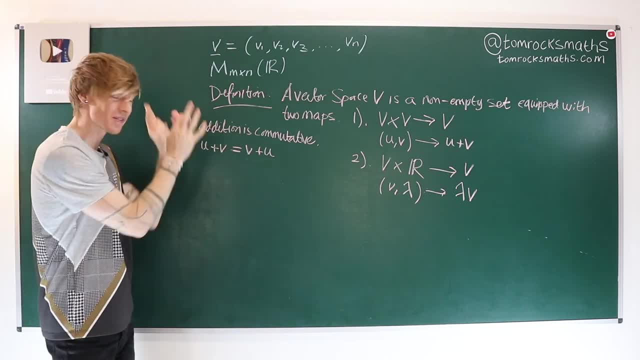 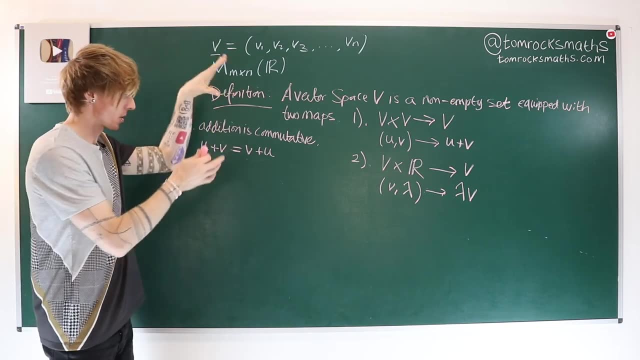 with real numbers and even with vectors, but we do need to define this as one of our rules or one of our axioms for a general vector space. And again, as I'm going through these rules, remember to always keep in mind our two examples of 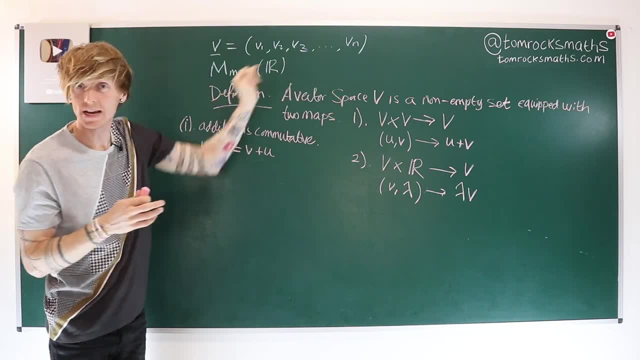 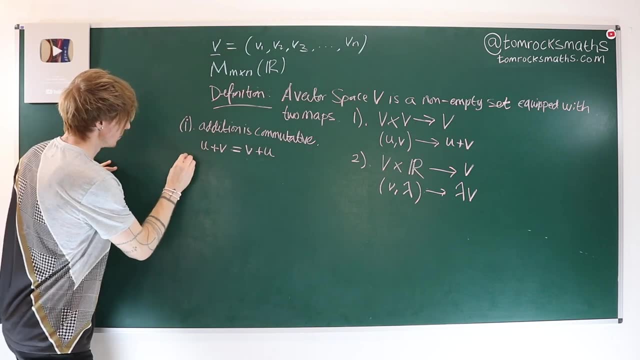 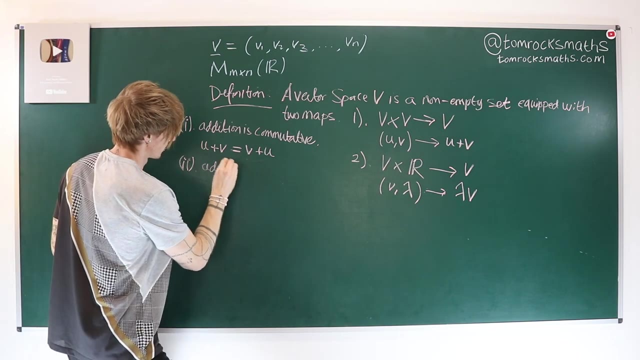 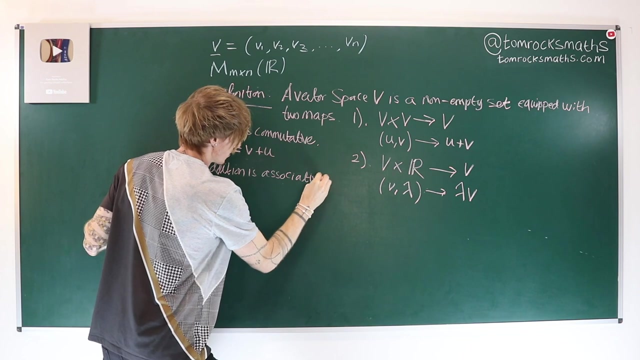 our n or n vectors coordinates with n entries and matrices. to really help visualize what these rules mean, Now a second rule is going to say that addition is also associative. Addition is associative. now, this one means that I have u plus v in brackets. 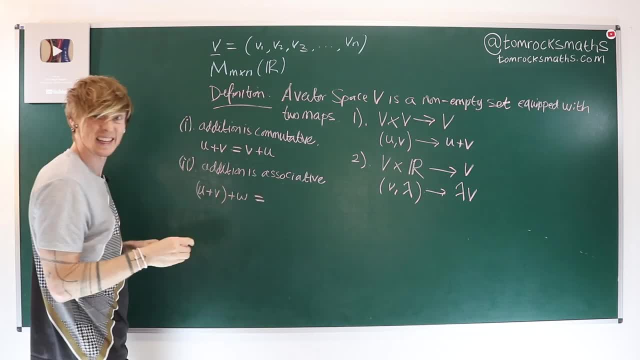 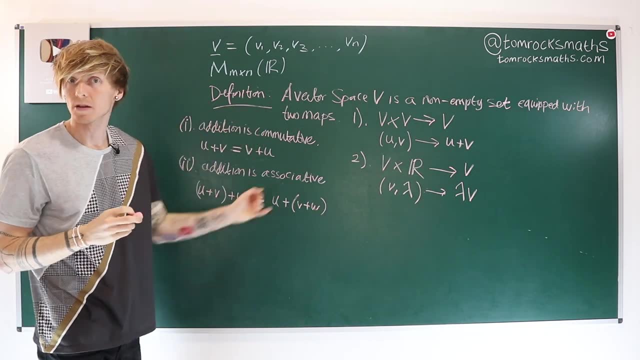 u plus v in brackets, u plus v in brackets. Now this means that I haveников brackets plus W and that's the same as if I did U plus first of all, adding V and W. So it's saying, if I add the first two and then the third one, or I add the, 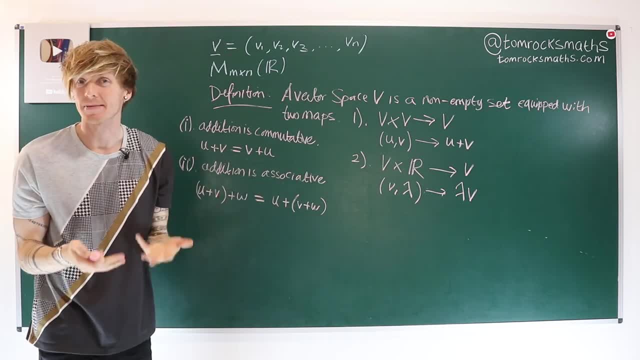 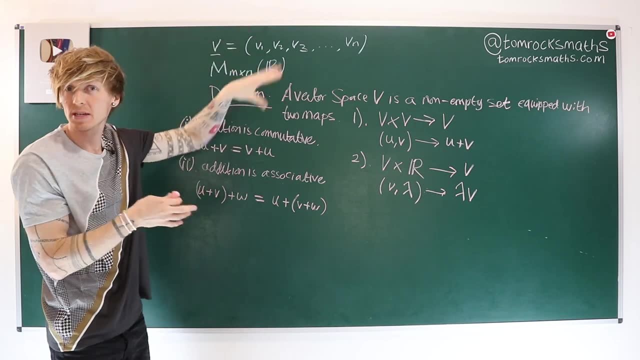 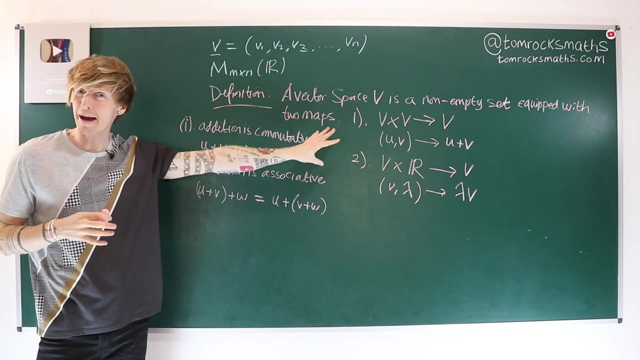 last two and then the first one. they're actually the same thing And, again, we are used to this. this is true in our number systems and our vectors and matrices that we're used to working with. Now, our third axiom says that the addition map. 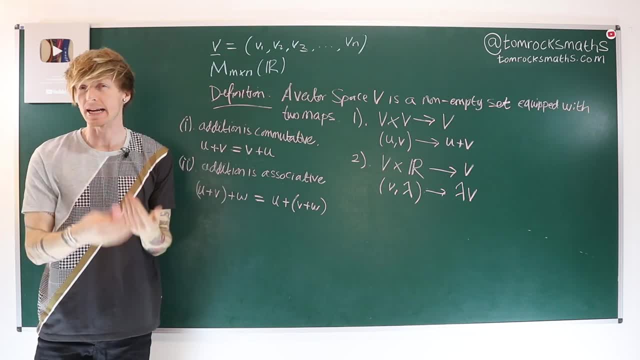 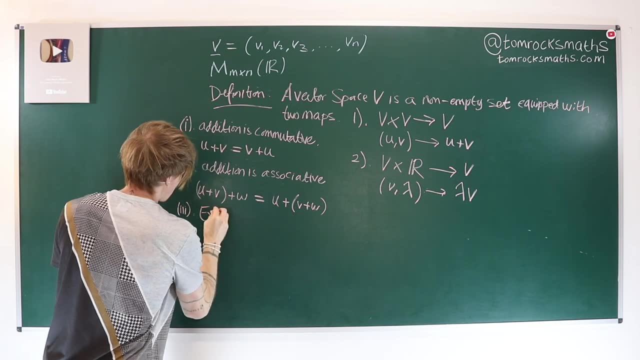 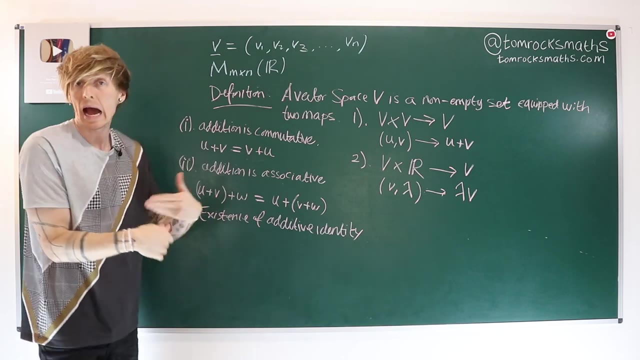 when we add together vectors, has an identity element. So this is going to be the existence of an additive identity. So what this means is that we have an element which I will label 0 for obvious reasons. we have an element which I will label 0 for obvious reasons. we have an element: 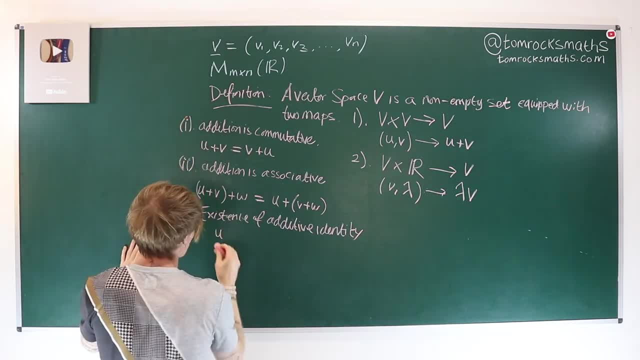 which I will label 0 for obvious reasons. we have an element that exists such that if I take a vector u- and this can be any vector u- and add the zero vector, which is going to be our identity element, then that's the same as doing zero plus u, and in both. 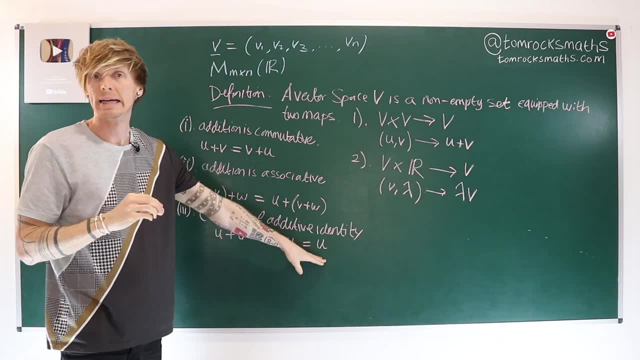 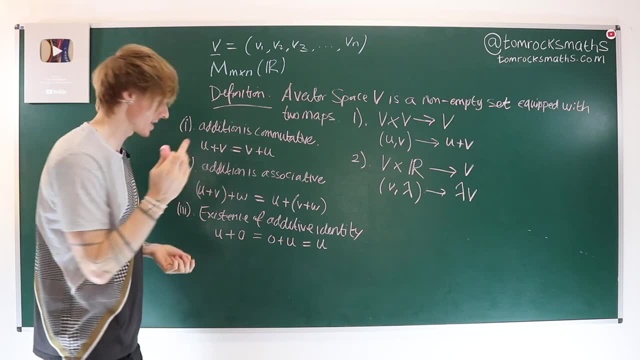 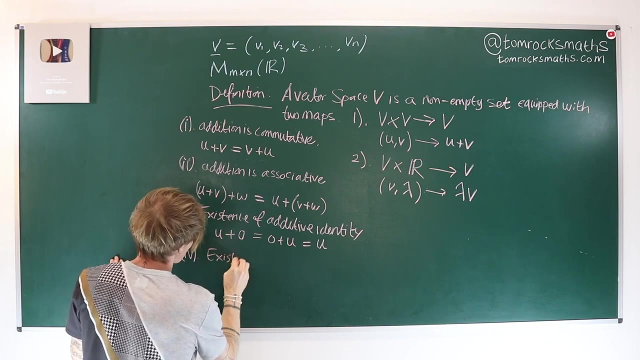 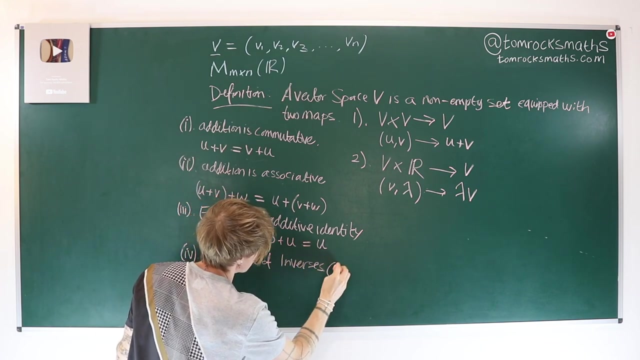 cases u is unchanged, I get back the same vector that I started with before adding the identity. And the fourth one actually follows from this really nicely. So the fourth axiom or rule tells us that we want inverses to exist. So this is the existence of inverses and these are going to be. 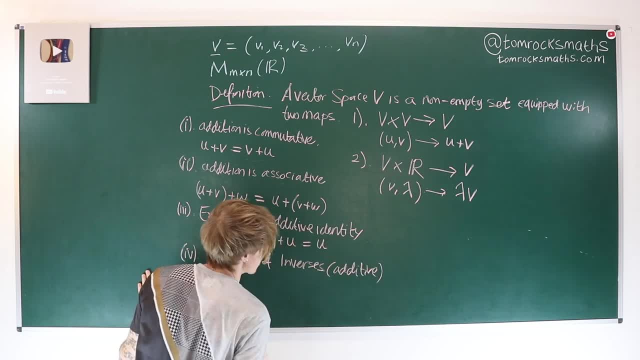 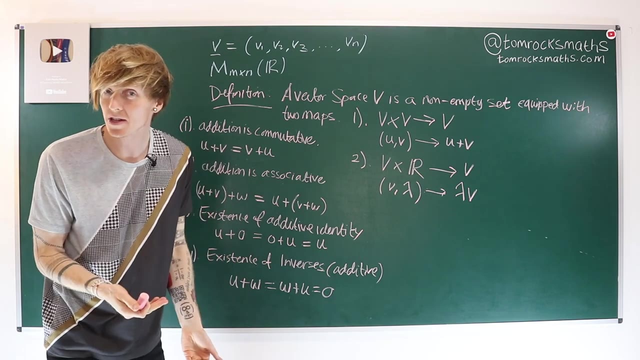 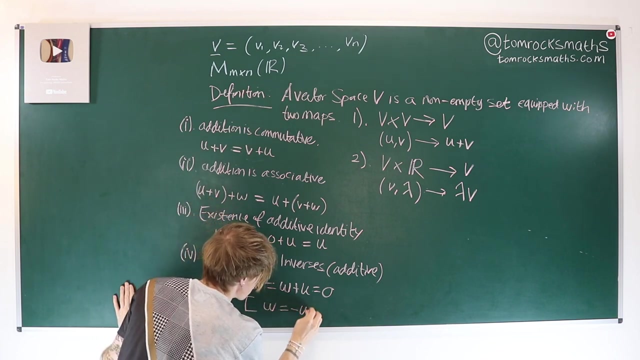 additive, again Just to stress that. So what's that going to mean is that u plus w equals w plus u equals zero, the identity element. So w is going to be our additive inverse, and I'll put this in square brackets Just to emphasize because some of you may have realized: w will of course be minus u. 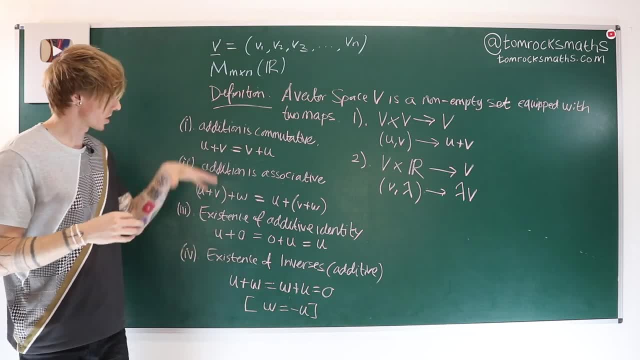 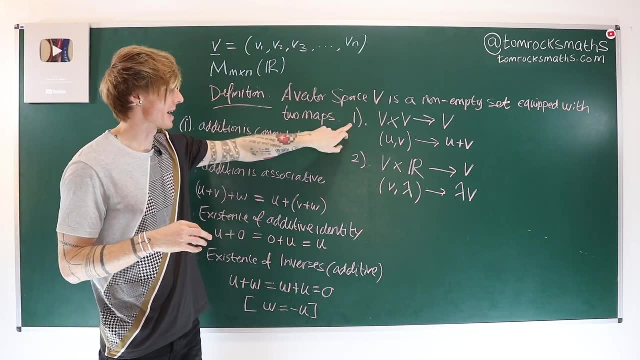 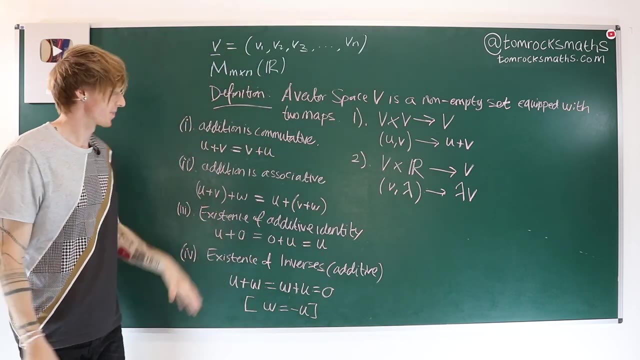 in the usual way. Now you may have noticed that so far the first four axioms all talk about the addition map which up here I labeled as our first map, where we take two vectors and add them together to get a new third vector. And these are all related to discussions about that. Now the final. 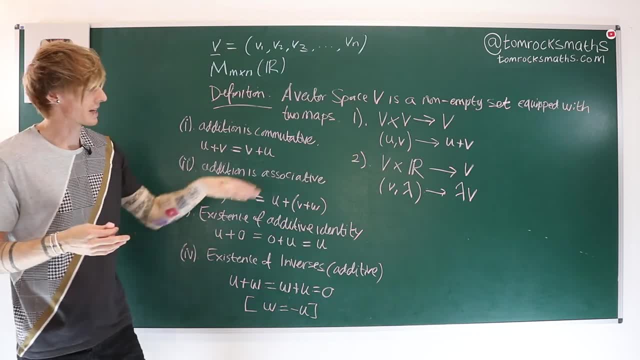 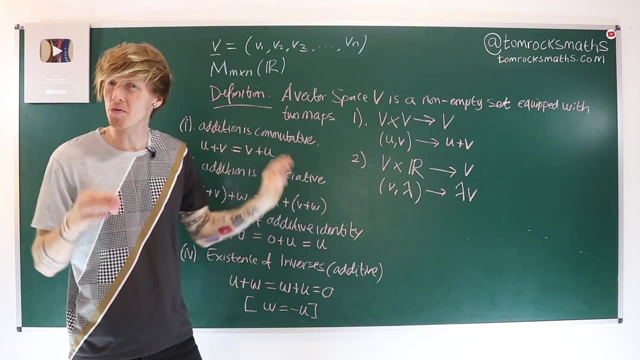 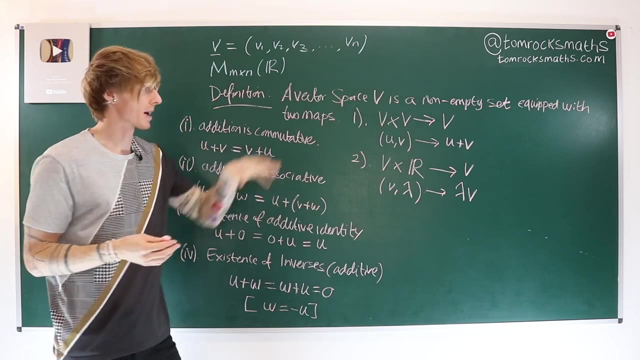 axioms are all about making sure that our second map of scalar multiplication. we want to make sure that this interacts appropriately with our vector addition. Now, exactly what that means will become clear when I write out the axioms. but there is an important distinction between these two sets. 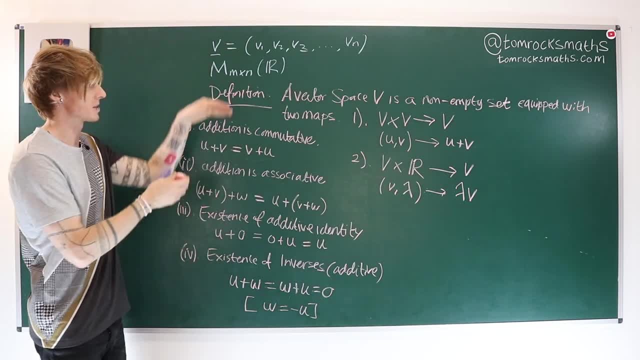 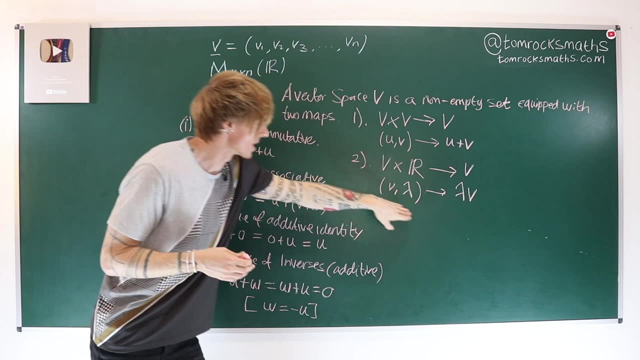 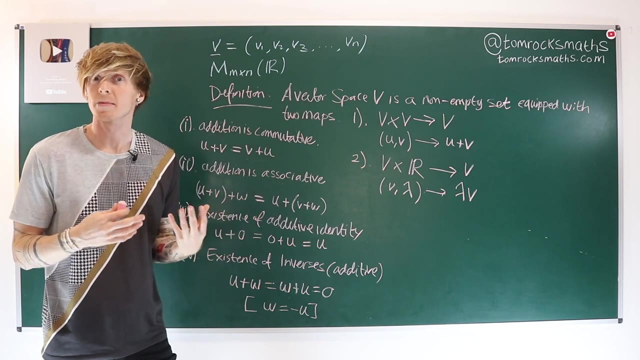 of four axioms. The first four talk about the addition map, where you add together the addition. The second four are all related to the interaction between the two maps, but in particular they focus on this scalar multiplication. The fifth axiom is called the distributivity of scalar multiplication. 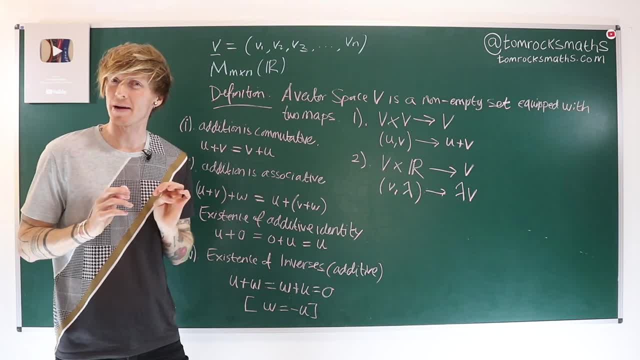 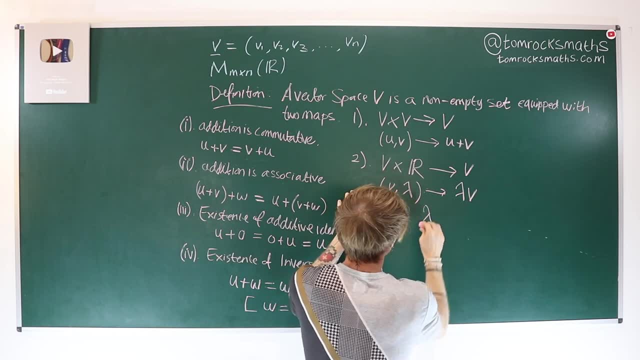 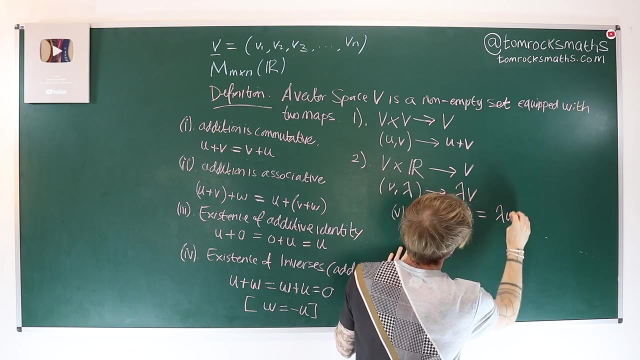 over vector addition, which is quite a mouthful. but what it means is the following: Our fifth axiom says that if I have a lander which will be a scalar, and that's multiplying u plus v, then that is of course going to be lander u plus lander v. And the reason I'm saying of course, 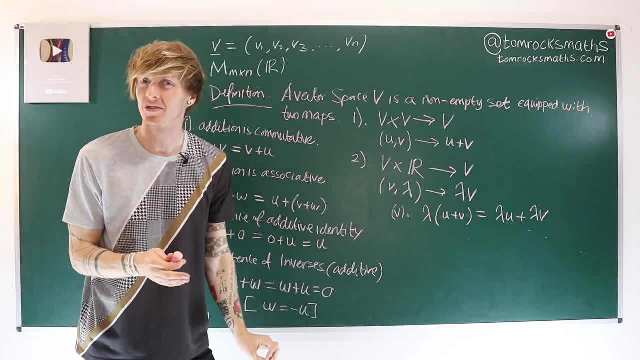 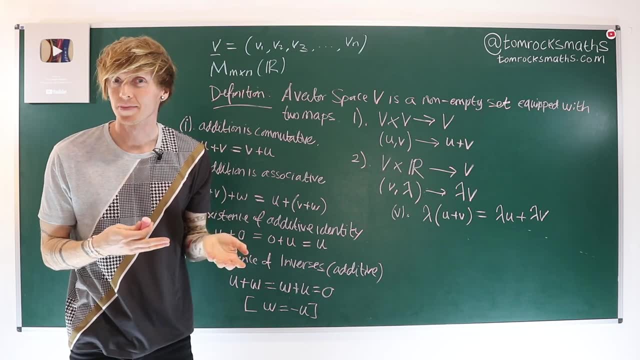 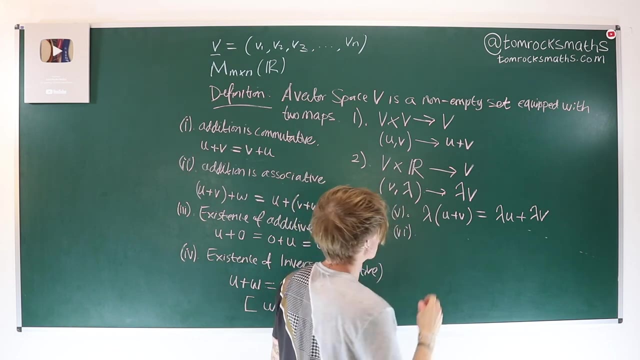 is because this is the definition we are used to. This is what we would expect with real numbers and the other objects that we're used to working with. Now we have a similar rule, which is going to be axiom six, which is going to be about distributivity again, but now we have lander plus. 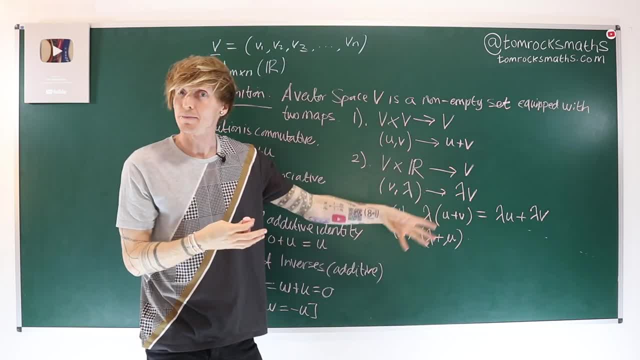 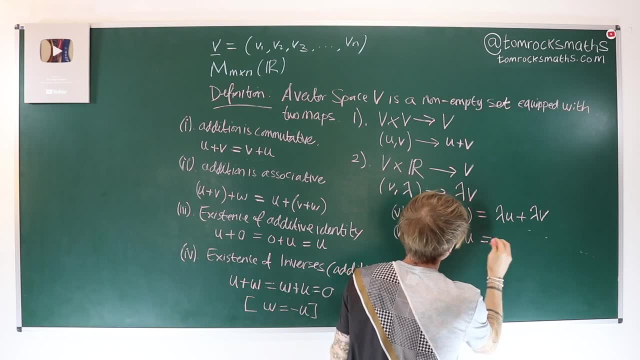 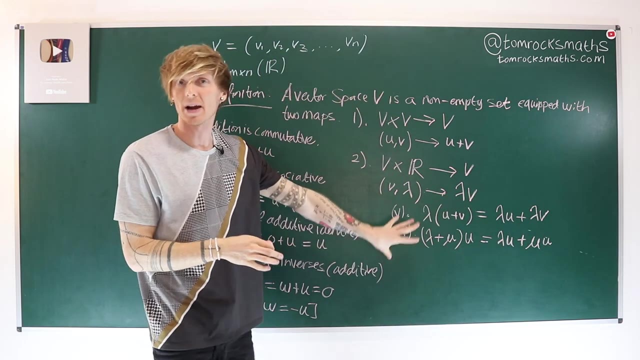 mu. So two scalar multiples, two elements from our field, which here is the real numbers added together times the vector u is of course the same as lander u plus mu times the vector u. So again you expand the brackets as we might expect. Axiom seven: 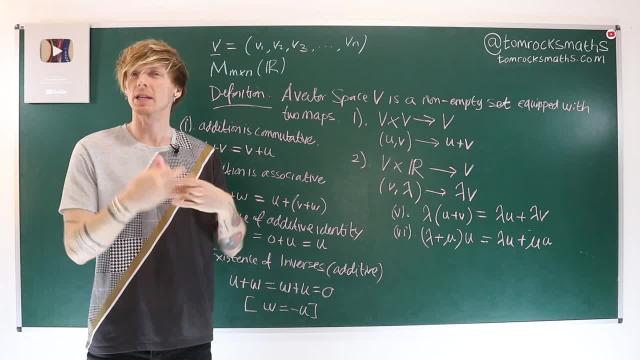 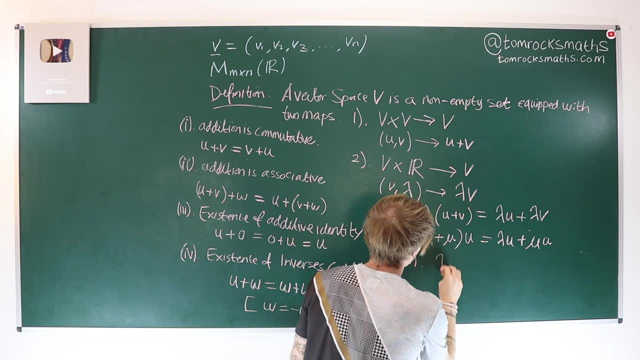 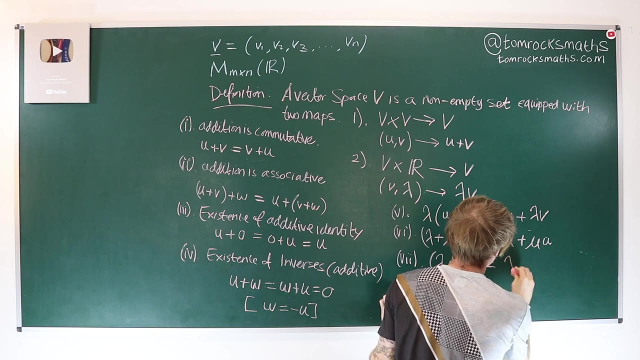 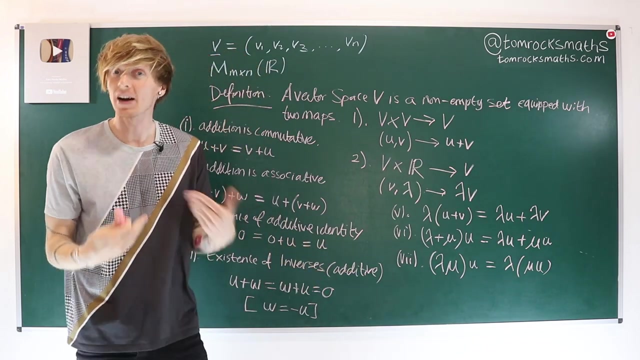 can be thought of as associativity for scalar multiplication. So what that's going to mean here is that if I have lander mu multiplied together times some vector u, then that of course will be the same as lander times mu u inside the brackets. And our final axiom, number eight, v, i, i, i. 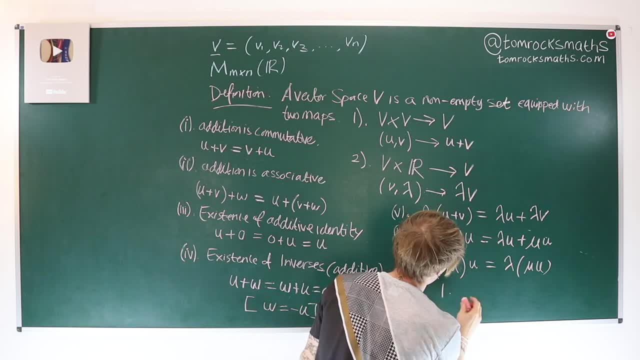 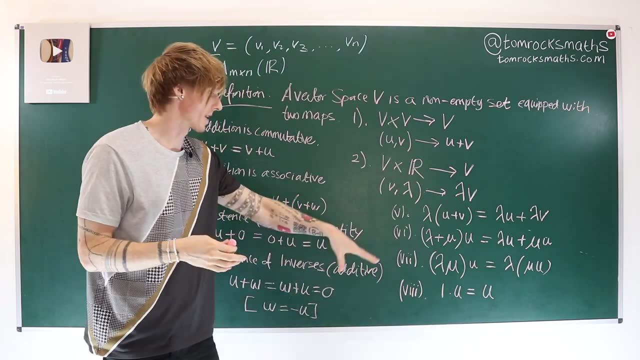 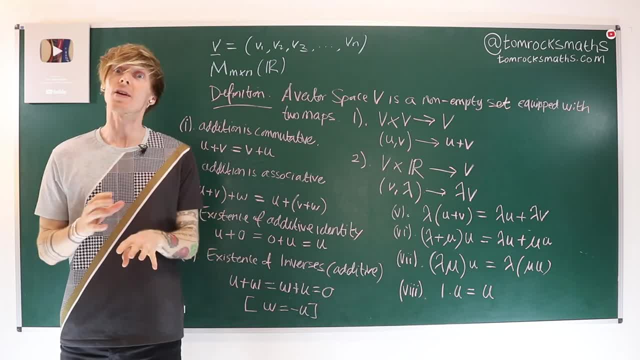 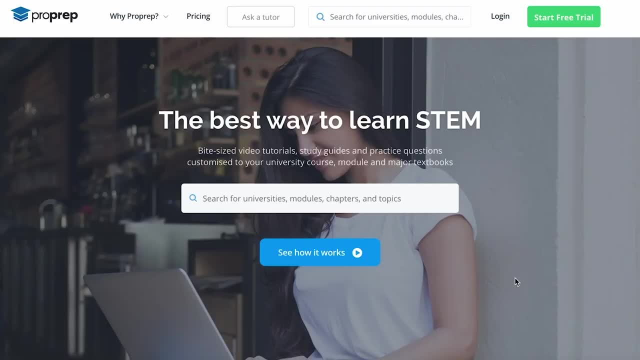 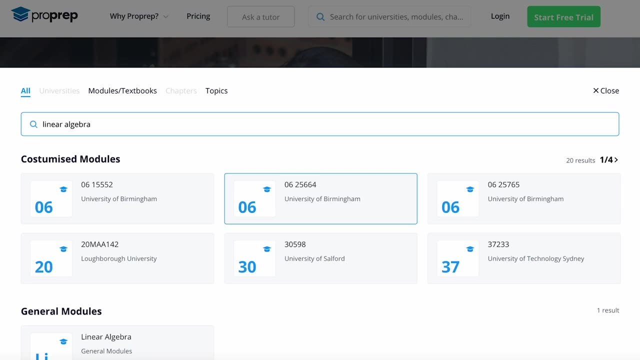 Now, before we look at some concrete examples, I do recommend checking out the teaching videos on ProPrep to really get to grips with the vector space axioms. ProPrep is an online resource that provides customized tutorials for students looking to improve their skills in stem-based subjects. 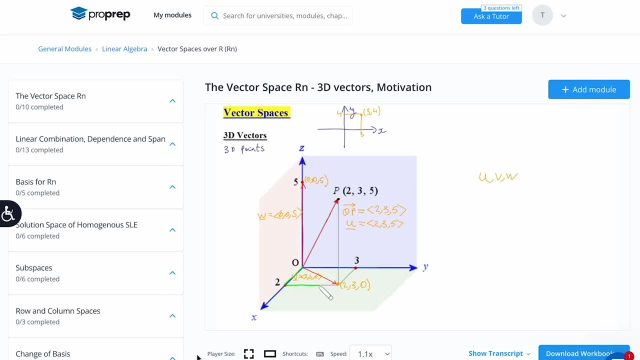 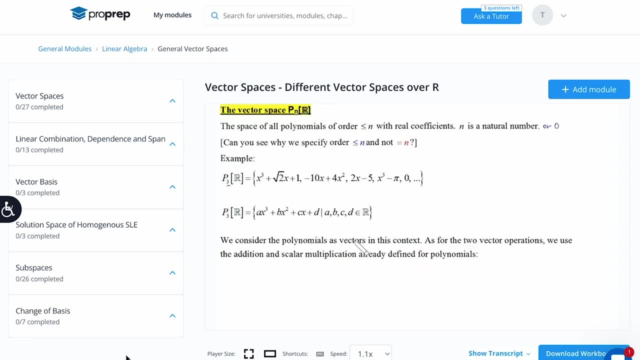 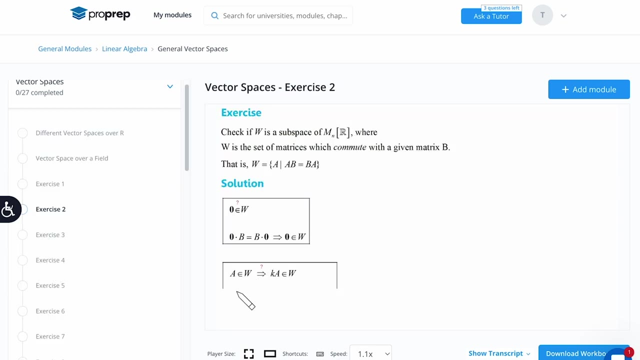 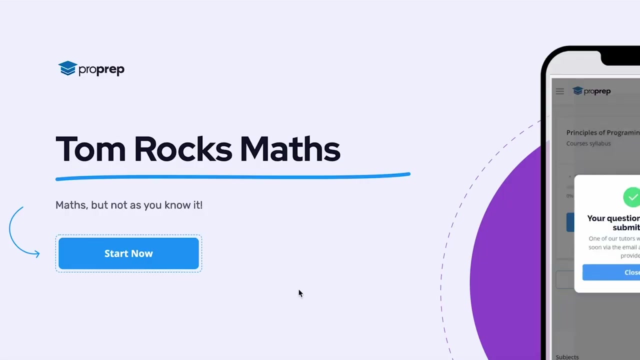 The videos on the vector space axioms are divided into two categories: first, looking at n-vectors and then progressing to more advanced examples with matrices and polynomials. As usual, each topic is accompanied by a series of practice exercises, each with their own video solution. so you can check your answer. Sign up for a 30-day free trial using the link in. 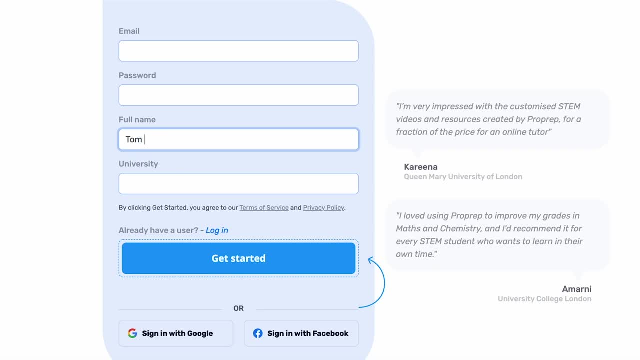 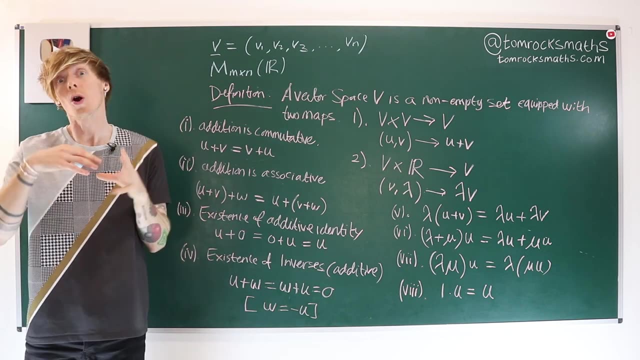 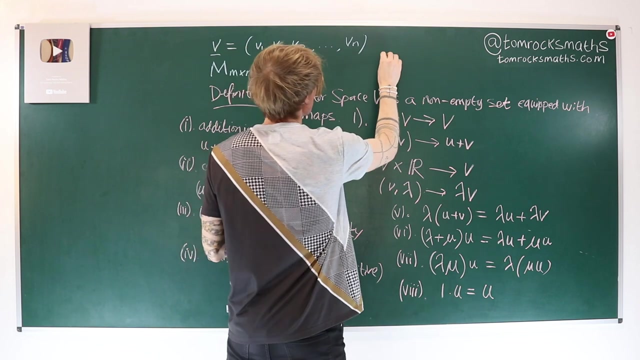 the video description to see how ProPrep can help you to improve your grades. Let's now look at a concrete example with three vectors. Three vectors or coordinates in 3D space. So if we take our general vector, let's call it v. 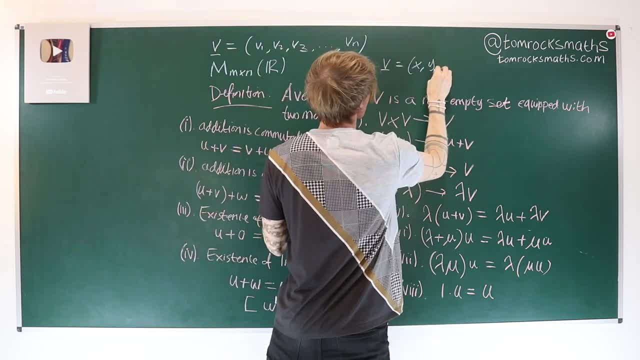 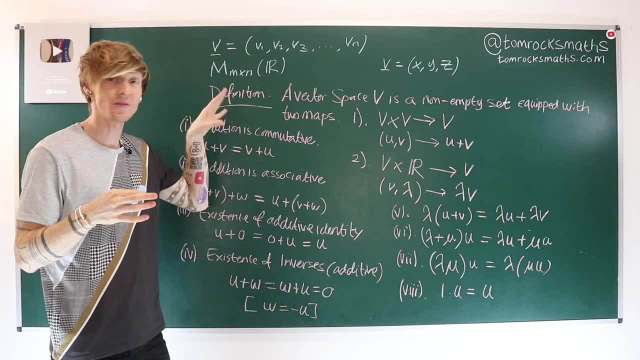 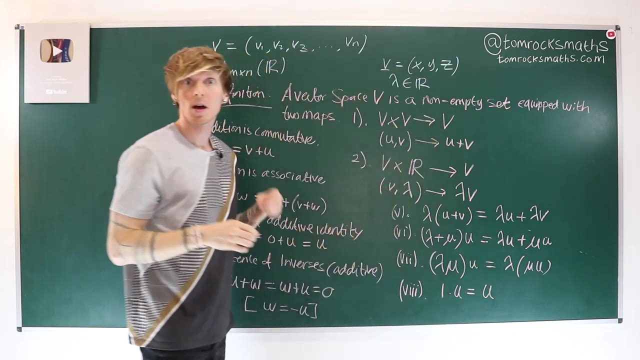 is going to be given by a coordinate vector- x, y, z- And, as mentioned in the definition of the vector space, our field is going to be the real numbers. so our lambda here is going to be some real number. Now, if we go through the axioms one by one, we'll see that the vector space axioms are: 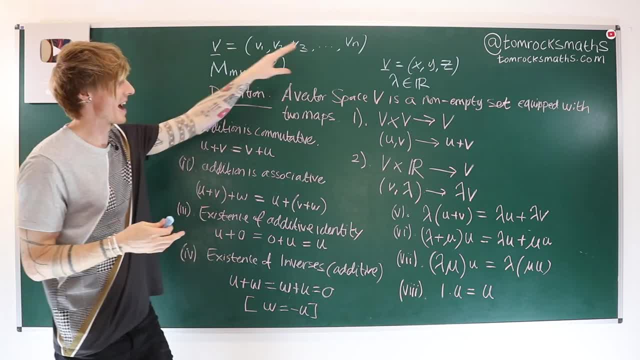 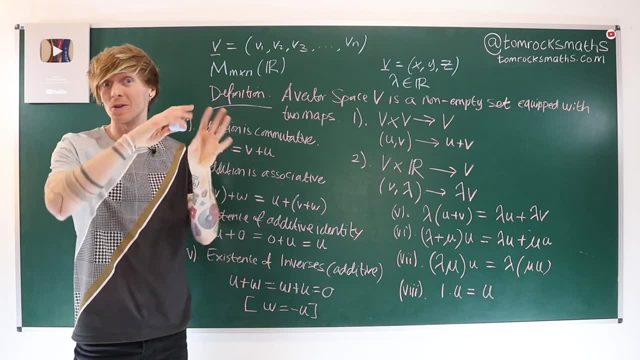 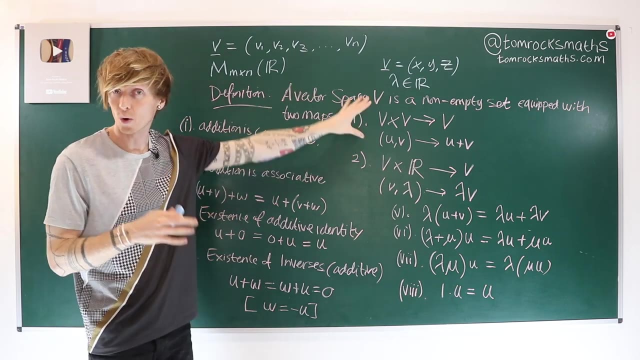 given by one, We can hopefully convince ourselves that this setup will satisfy all of these axioms and therefore we have a vector space which will be our 3D coordinate system. We start by checking that the maps defined here, one and two, make sense. 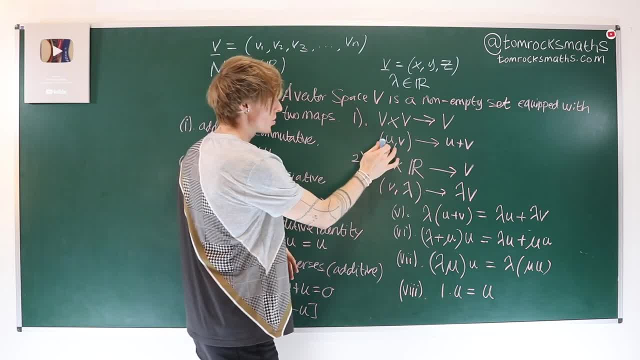 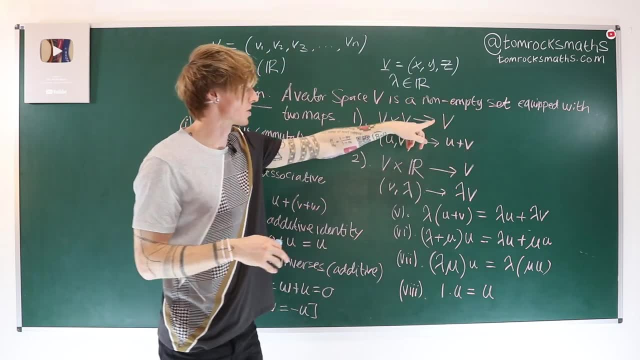 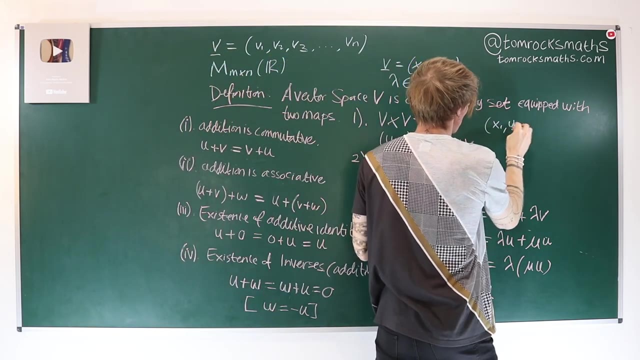 So the additive map says that if I take two vectors in my space and add them together, I need to get a third new vector Which is also in the vector space. So here that means if I take x1,, y1, and z1, 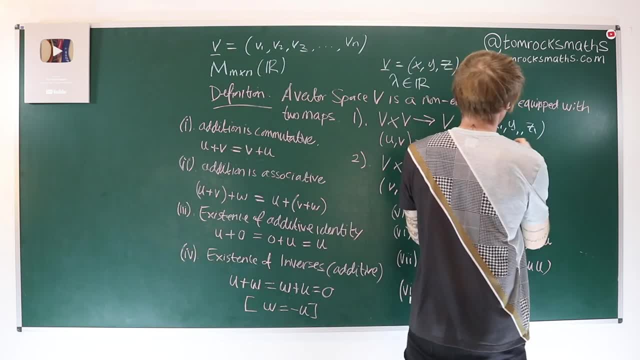 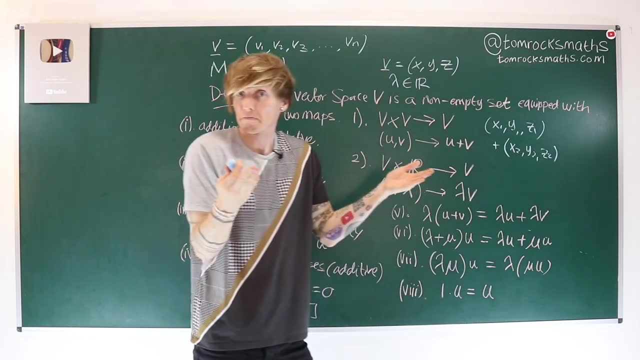 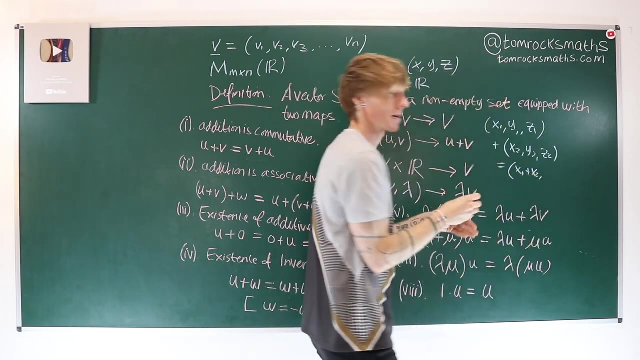 to be a point in 3D space and then I add a second point, so let's call it x2, y2, and z2, then hopefully you can clearly see that I will end up with x1 plus x2.. We add together. 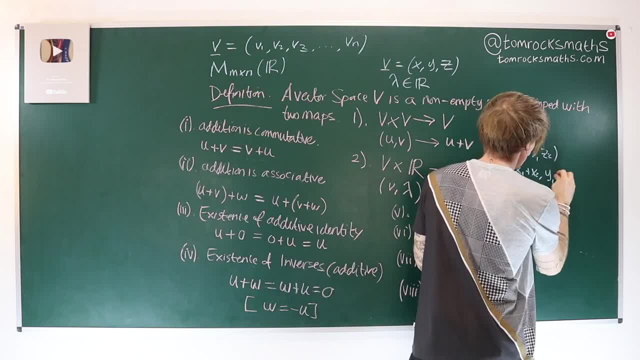 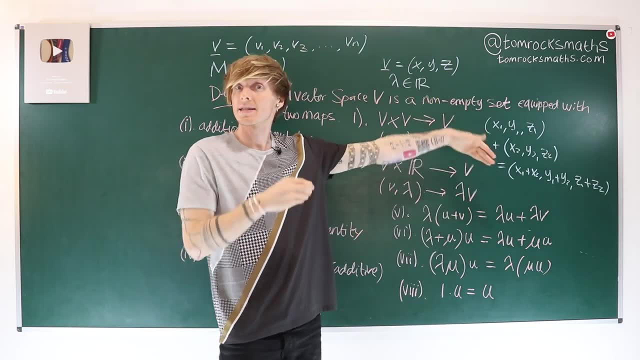 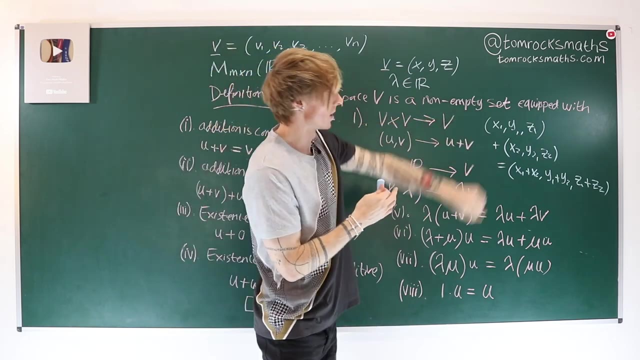 the x coordinates, We add together the y coordinates- y1 plus y2, and the z coordinates gives us z1 plus z2.. Now this is still going to be a point in 3D space. So we started with two points in 3D space. we added them together. 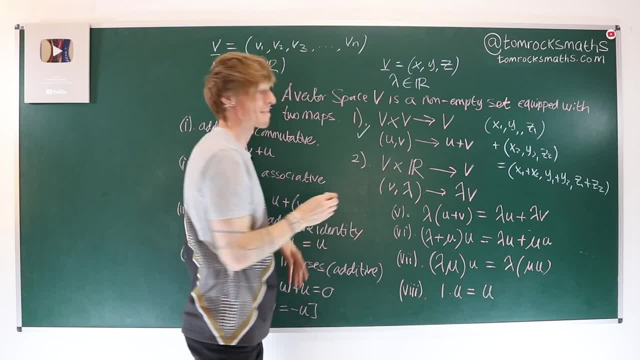 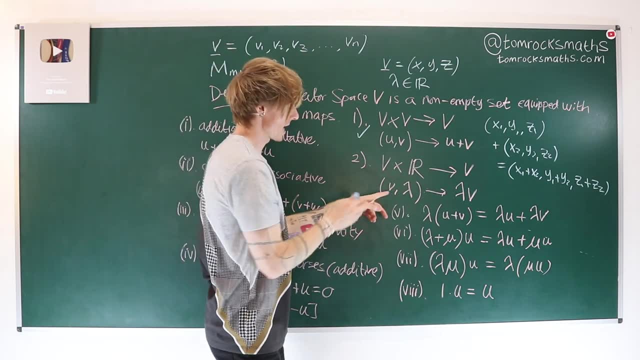 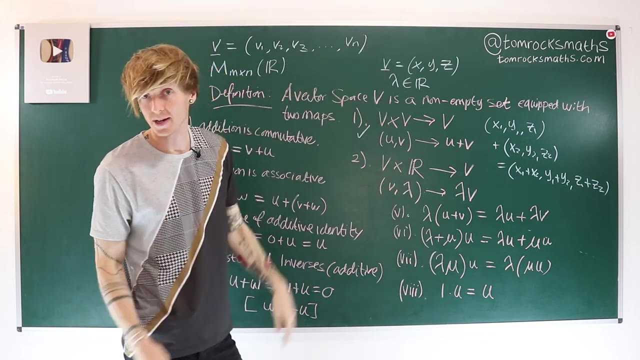 we get another point in 3D space, This map. it makes sense. Now for the scalar multiple map, we need to take a lambda, which is a real number, and a coordinate vector, which up here is x, y, z. 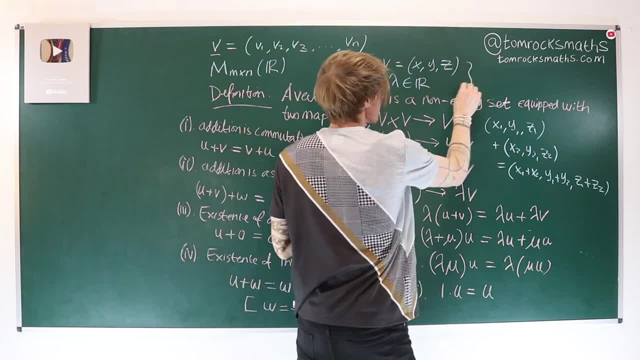 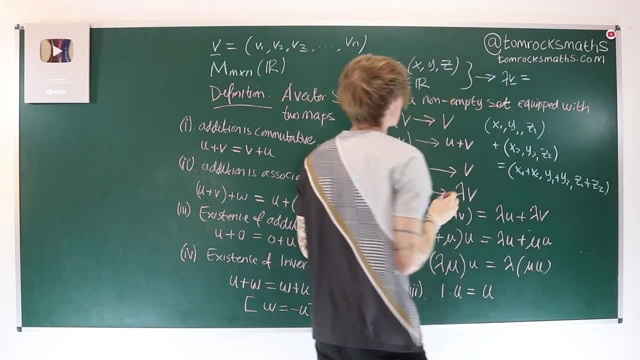 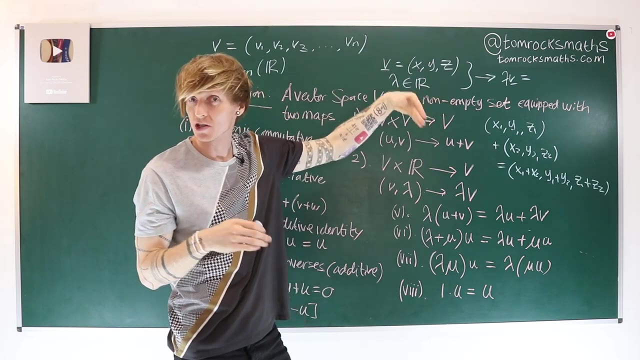 And then we multiply them together. So, based on this, we can say: lambda times v. lambda times v is therefore going to be lambda, multiplying each individual position or each individual coordinate across the whole vector, because that's how scalar multiplicators 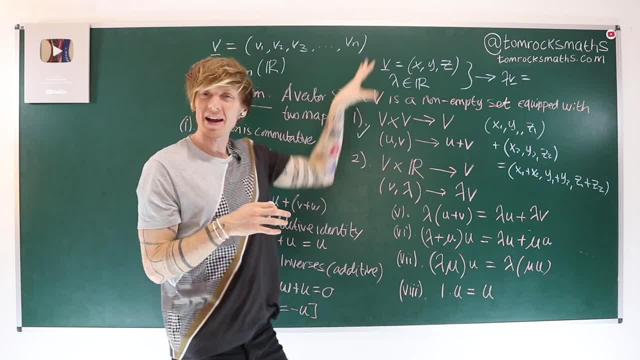 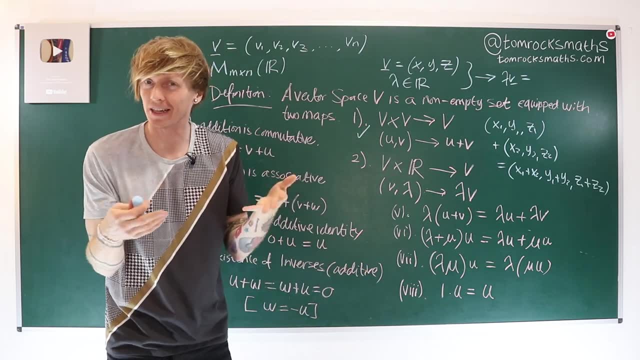 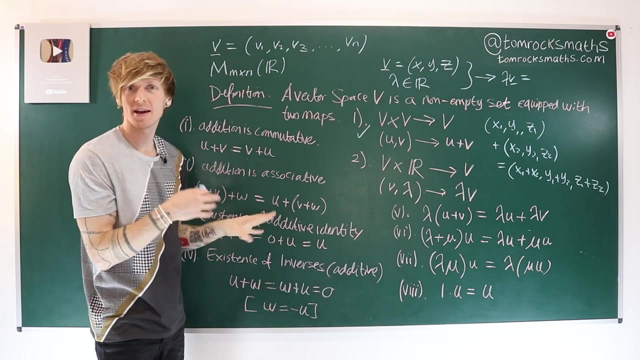 or scalar multiplication of a vector works. Now, this might feel sort of obvious, but it is important to check this, And the only reason it potentially feels a little obvious is we are used to working with vectors and that's why I said it's helpful to think of them. 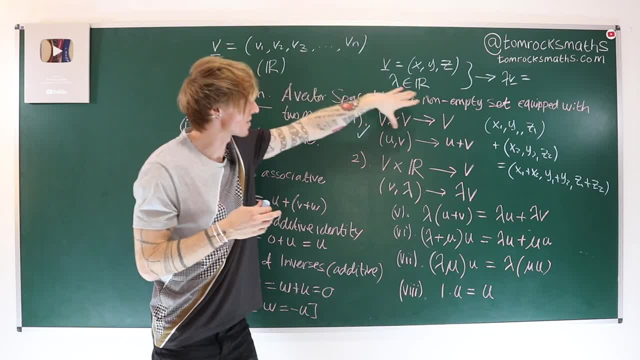 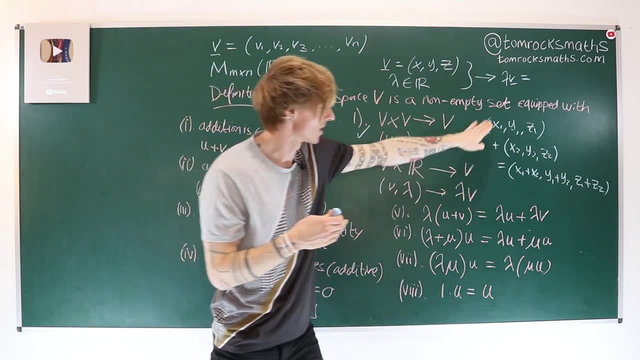 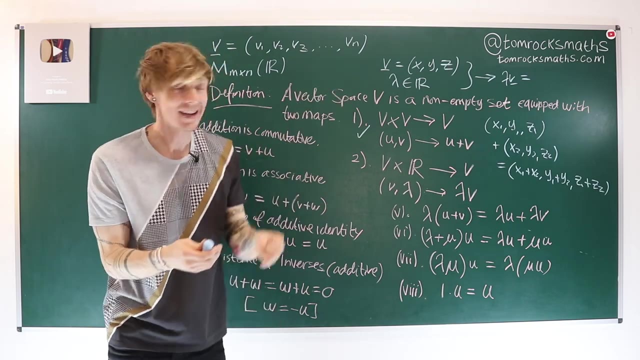 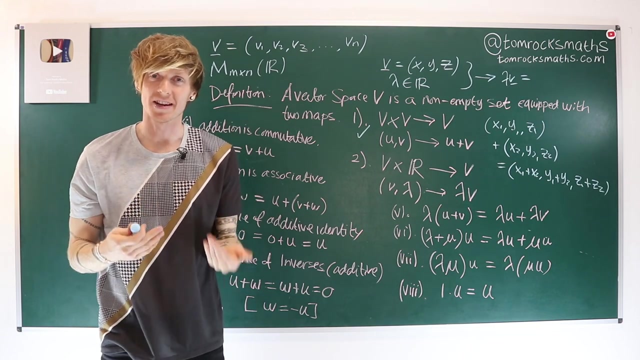 as our canonical or concrete example. But the reason we defined scalar multiplication of a vector or vector addition, where you only add together corresponding coordinates- the reason we defined those operations in the way we're used to is precisely to make sure that vectors fit within the vector space definition. 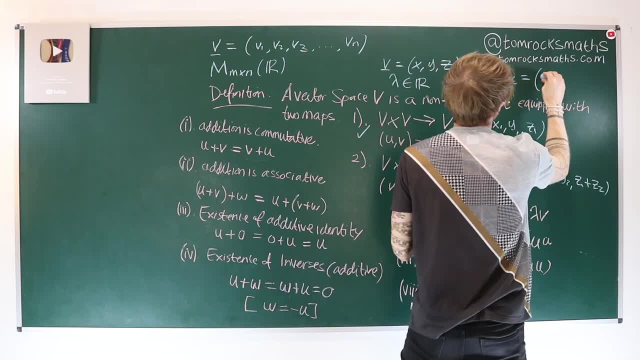 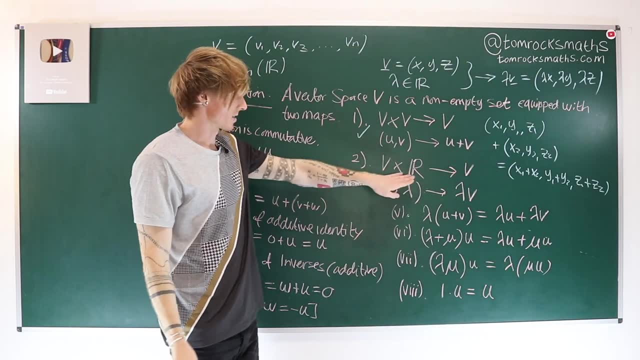 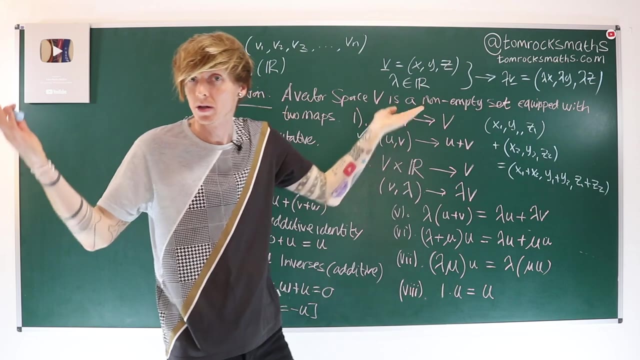 So proceeding. we can say: lambda v is then just lambda x, lambda y and lambda z. Okay, and that is of course within our original vector space. If I have a coordinate, multiply it constant, say it's two, say lambda's two, I get a new position that's further away. 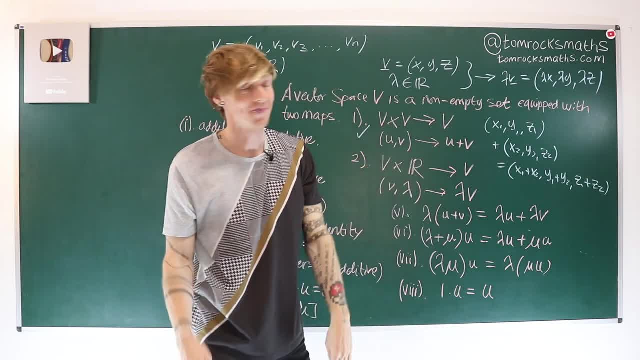 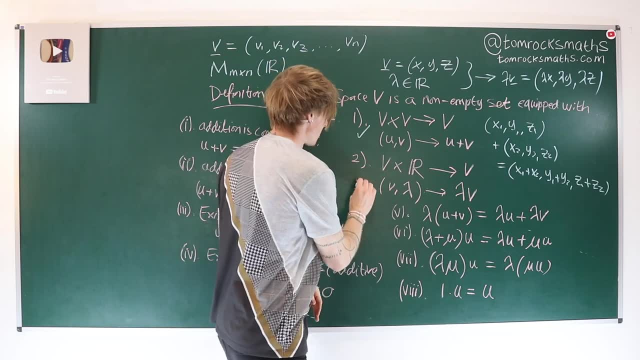 It doesn't have to be further away. lambda could be. a half makes it closer to the origin, But either way, what we're going to do is get another point in 3D space. so we do indeed have a map that is mapping into or moving into the correct vector space. 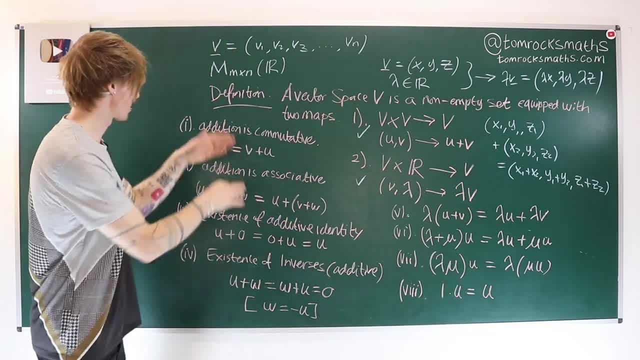 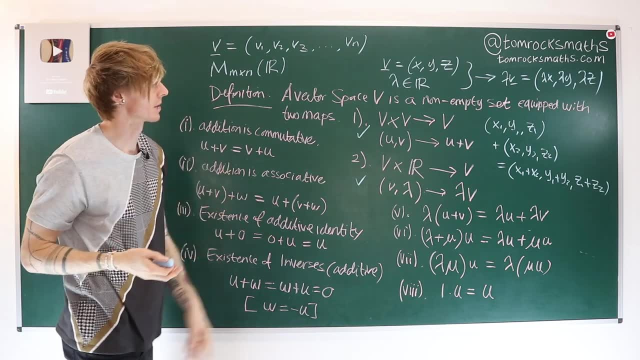 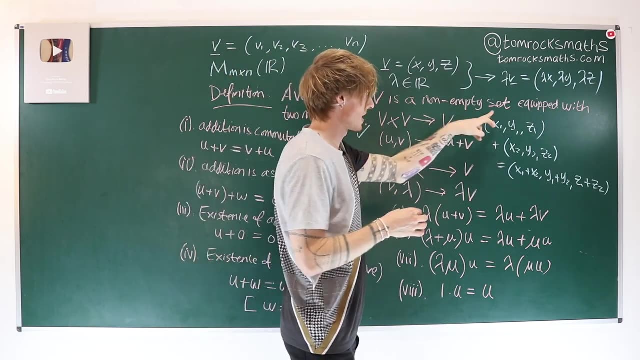 Now going through the axioms themselves one by one. we start with: addition needs to be commutative, which says I can add together two vectors in any order. So if I take my three vectors over here, the first one can be u, the second one can be v. So when I add them together, 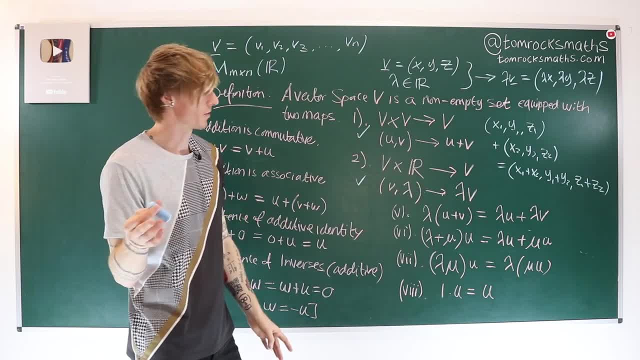 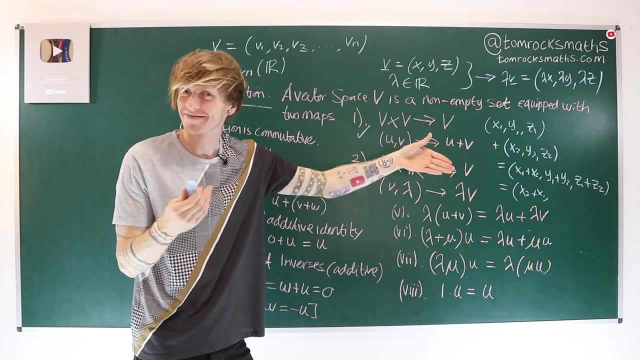 I could get x1 plus x2,, keeping them in order, But of course that's exactly the same as x2 plus x1, because each individual entry is a real number: y2 plus y1, and z2 plus z1,. 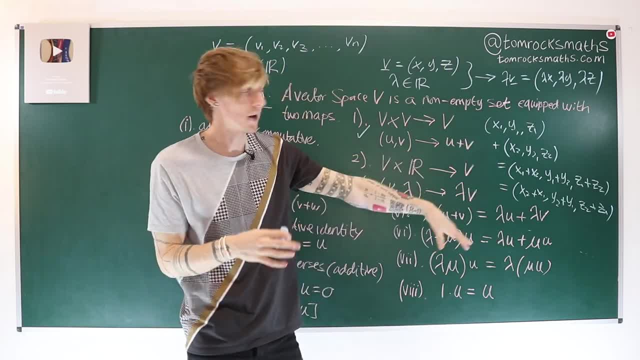 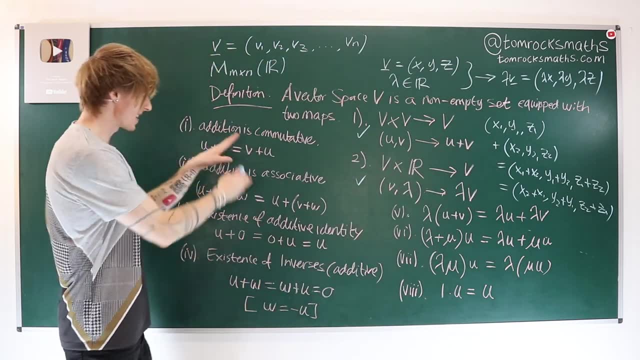 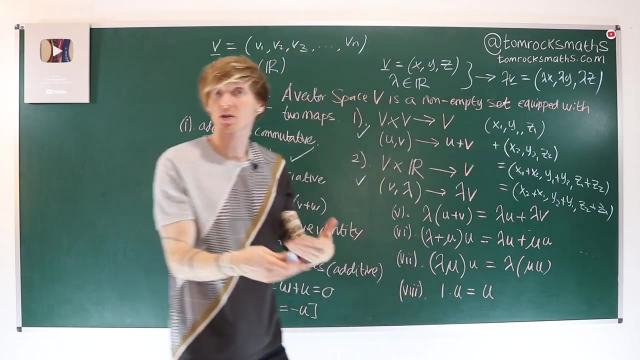 and so that sort of breaking it up into its components is just the same as adding the one with the twos first to the one with the subscript one. So we can see that this is indeed going to work. It doesn't matter in which order I add my two three-dimensional coordinate vectors. 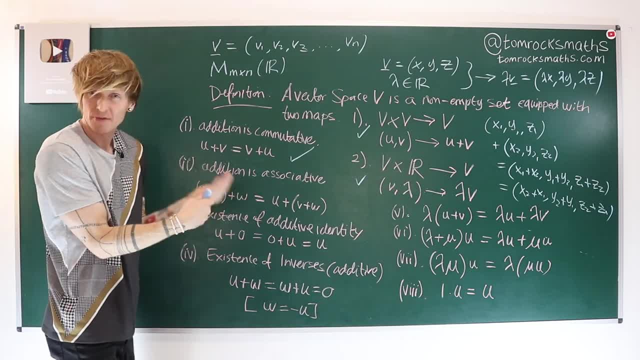 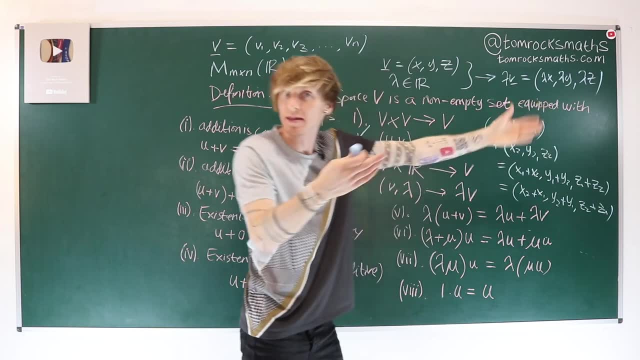 Now for associativity. again, it follows in a similar way. If I add together the first two and then add the third, I end up with a vector with three things added in each position. And then, if I add the second, two, 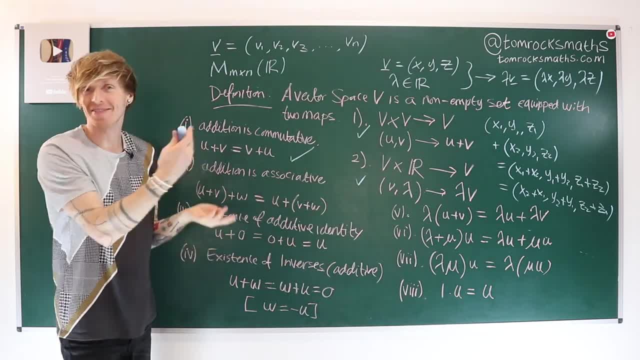 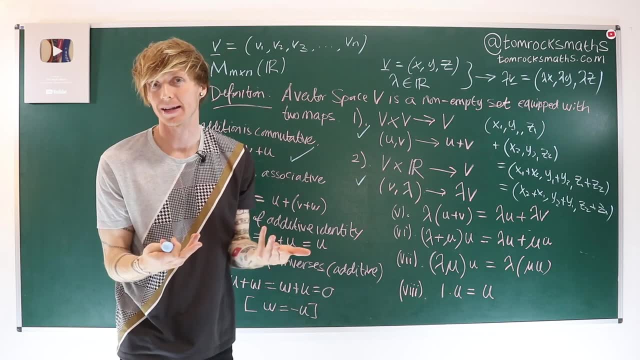 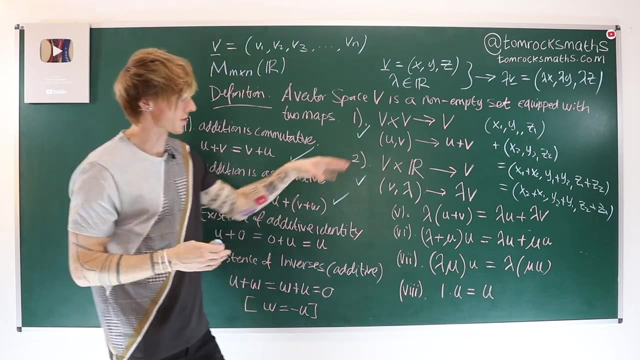 and then go and add the first one, I still end up with a vector with three things added together in each position, and the order of those three things of course doesn't matter. So hopefully you can see that associativity is also going to follow, just because of how we define this addition of two vectors. Now the third one. 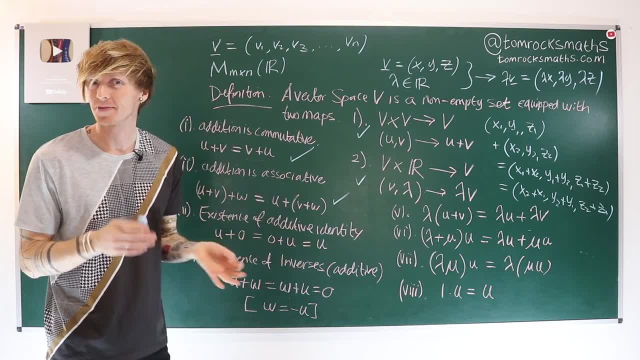 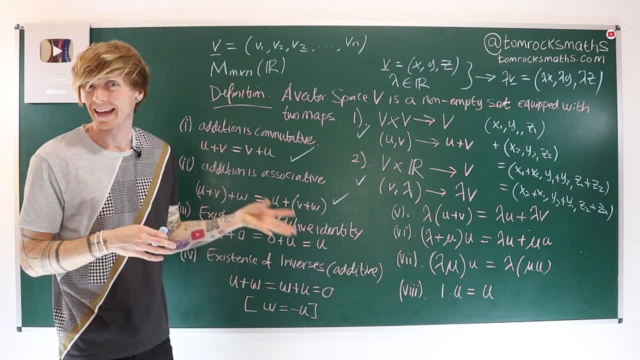 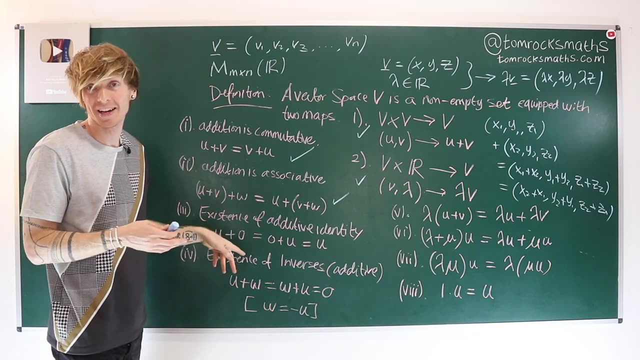 talks about the existence of an additive identity, So we do need to think a little bit here, because we have to identify what this identity element is. in the case of three-dimensional vectors, The clue, of course, is in the fact that I labeled this the zero vector. So the zero vector. 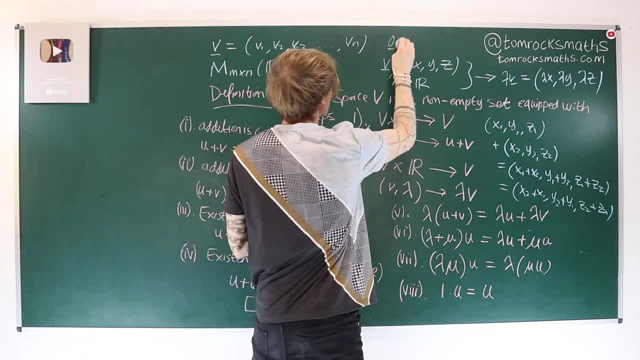 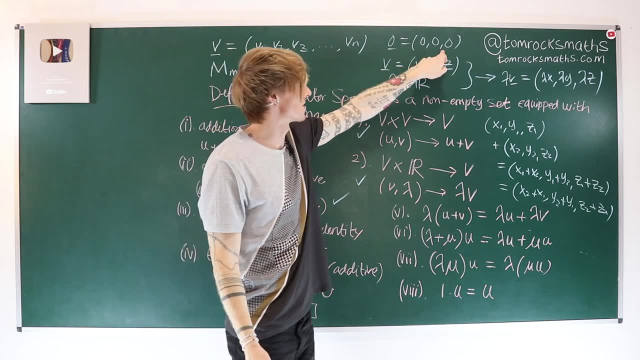 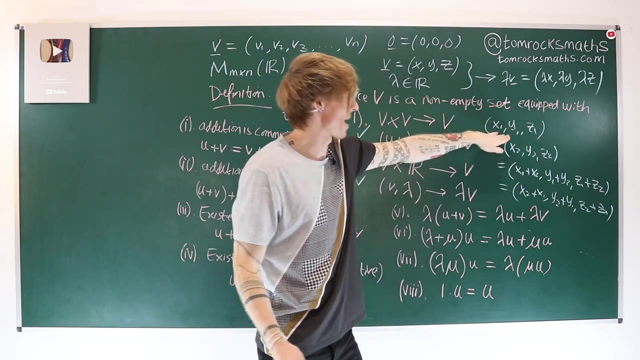 in the case of three dimensions, is simply going to be zero, zero, zero. So if I have the zero vector, three lots of zero. if I were to add them in here, this would be zero, this would be zero, this would be zero. you can clearly see. I'm just going to get back exactly what I started. 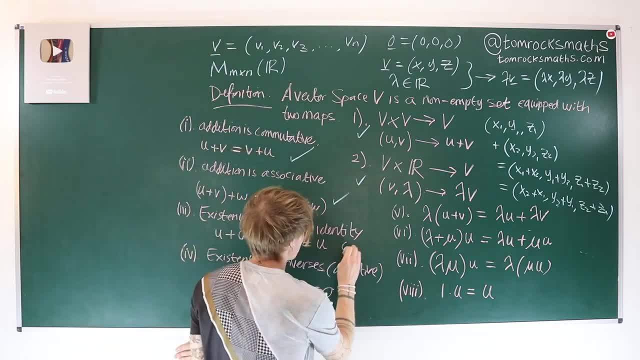 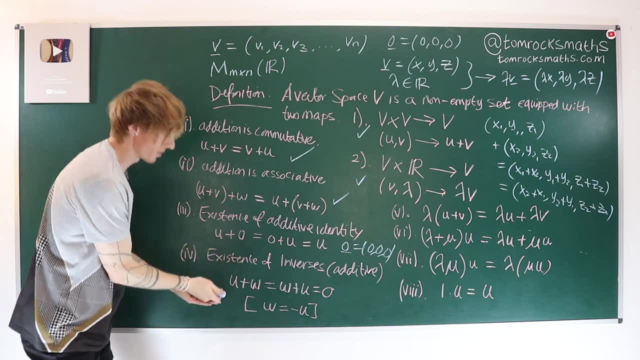 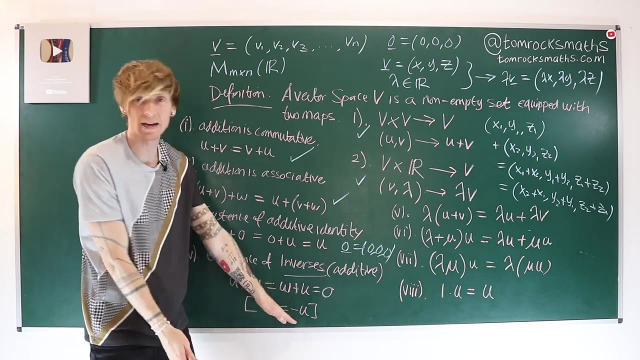 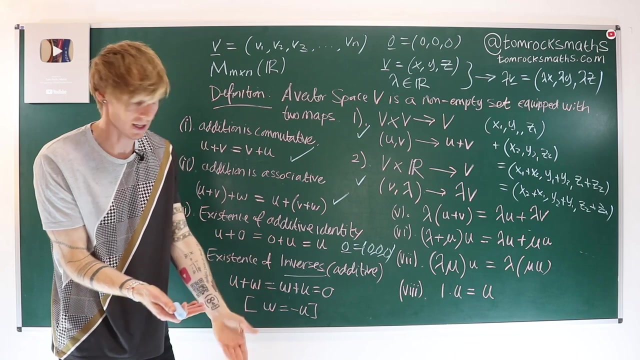 with. So we do indeed have an identity, which here is zero, zero, zero. And again, for the fourth one, we need to identify what the inverse element looks like. So again, we need this w, which can also be written as minus u. We need this element such that when I add it to u, a general vector I need to 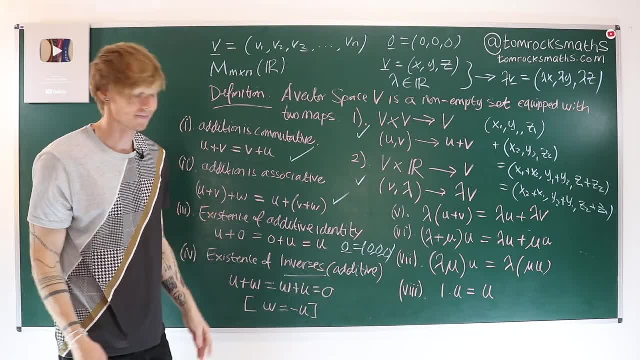 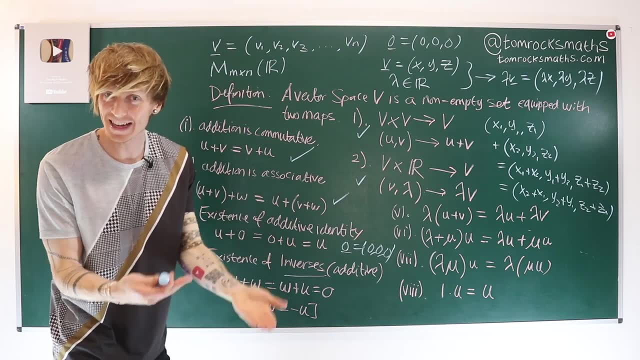 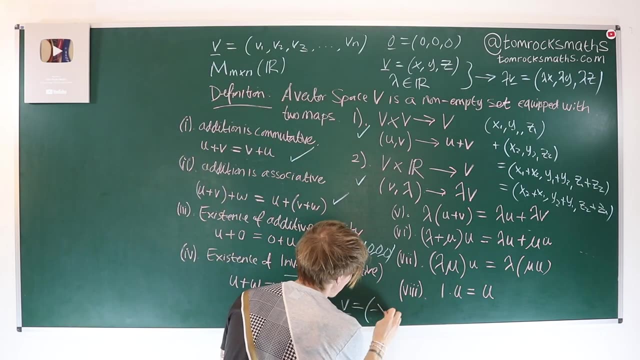 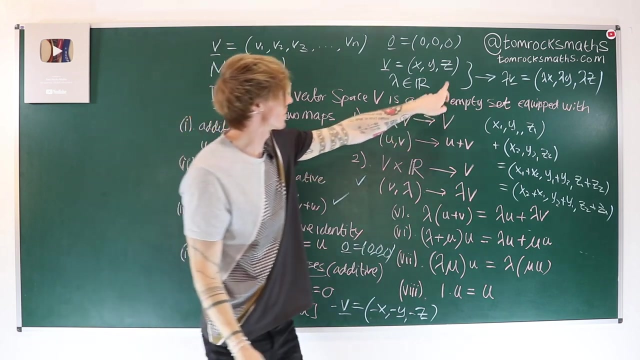 get zero because zero is our identity. So here, if I have my general vector x, y, z, then the additive identity, or minus, that is simply going to be minus v, which is going to be minus x, minus y and minus z. If I now add this to my original v, I'm going to get zero, zero, zero, which is the identity element. 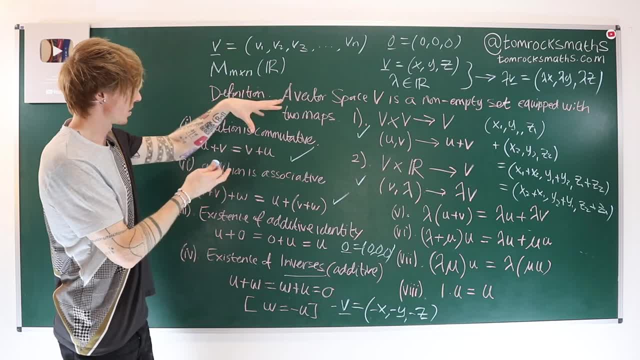 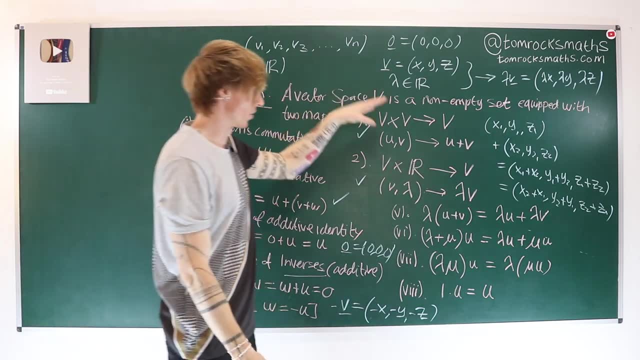 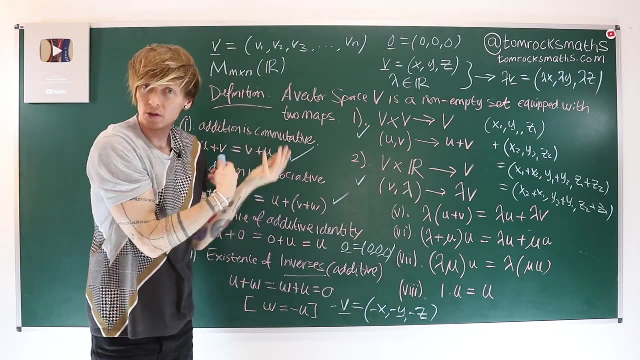 So that completes the first four axioms talking about the first map on addition of vectors. For the second four, labeled from five through to eight, again we're going to have to just check that our usual way of working with three-dimensional coordinates is going to. 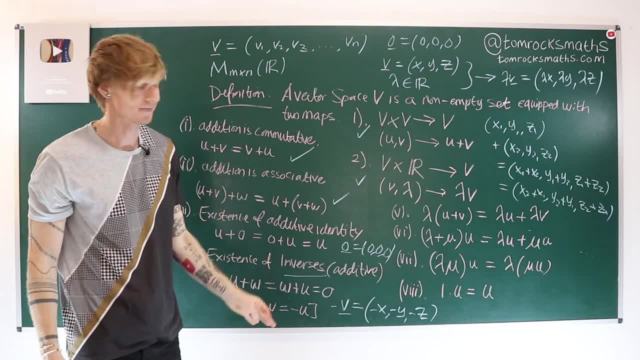 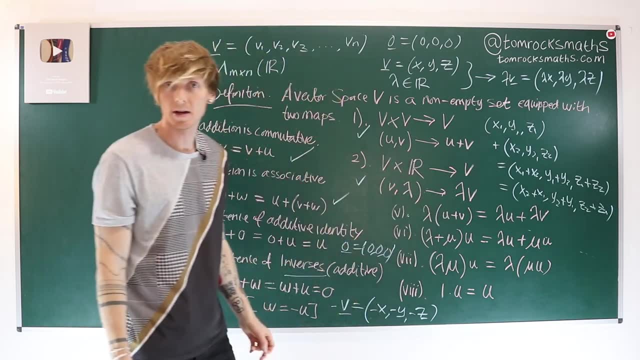 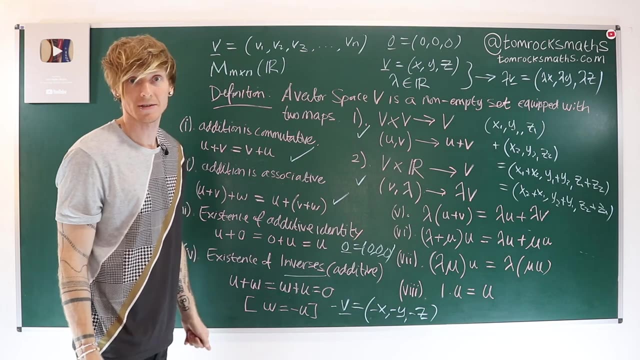 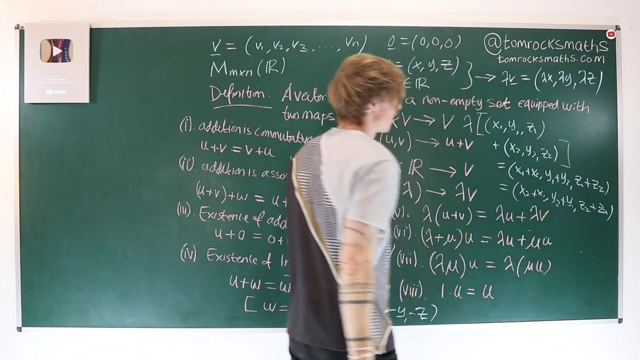 make sense in this context. So I have a number, real number, lambda, multiplying the sum of two vectors, and that needs to be the same as lambda times the first plus lambda times the second. So I can go in and say, okay, so if I have a lambda here multiplying that one plus, 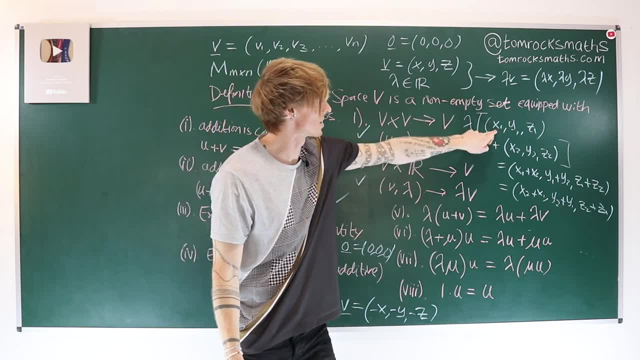 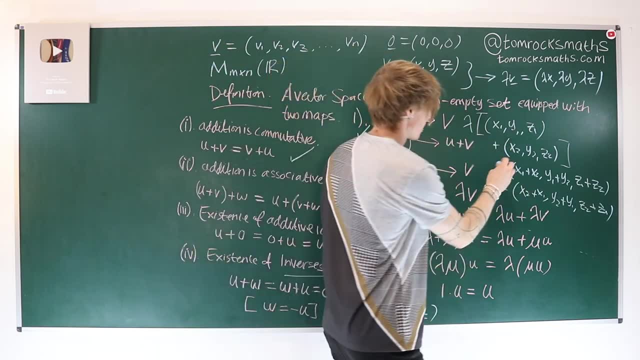 that one. so that's lambda times u plus v. This is lambda, this is u and this is v. So if I were to do that, I can add them first, and then I'd still have a lambda outside, and then I can, of course, take the lambda inside. So if I now replace all of these, 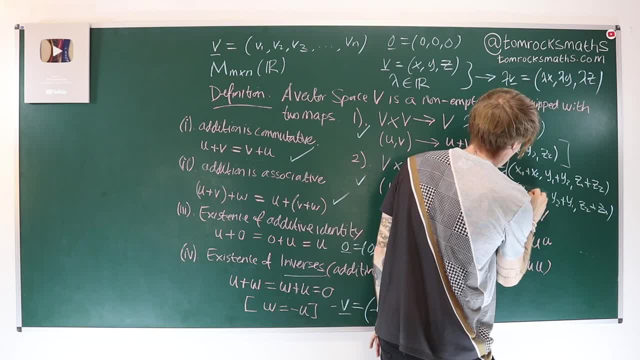 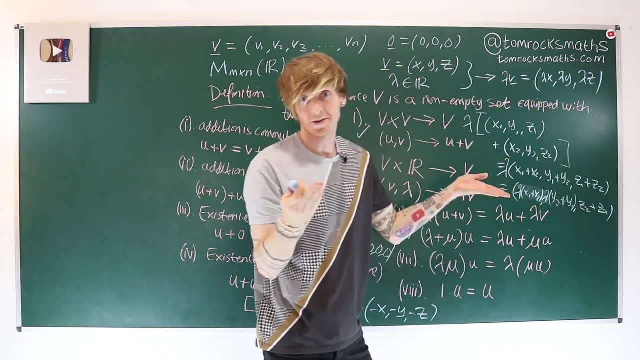 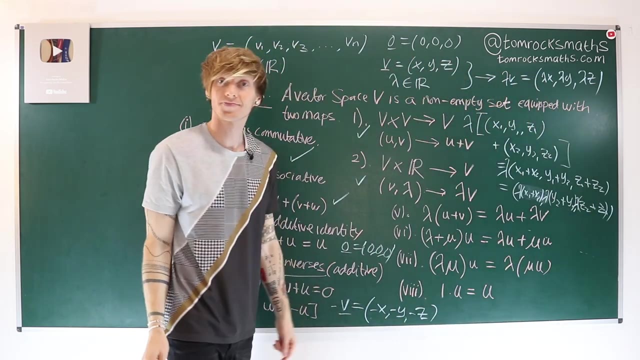 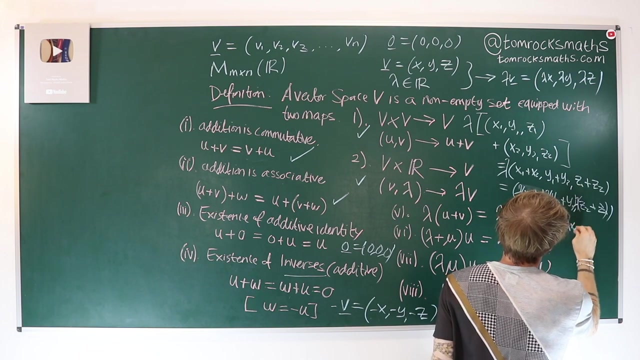 with the lambda definition. now I'm going to have lambda times x1 plus x2, lambda times y2 plus y1, of course the order doesn't matter, as we've already established- and lambda times lambda z. Now I can expand out that bracket and say: well, that's just the same as lambda x1 comma. 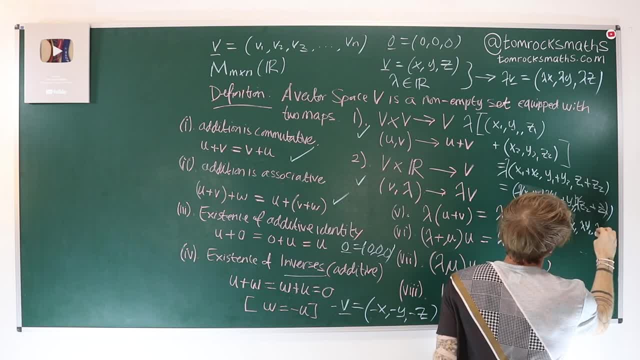 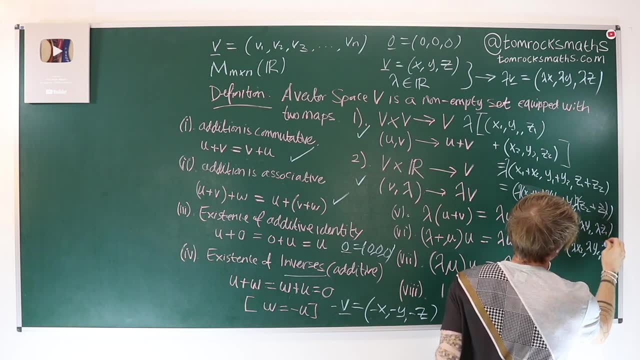 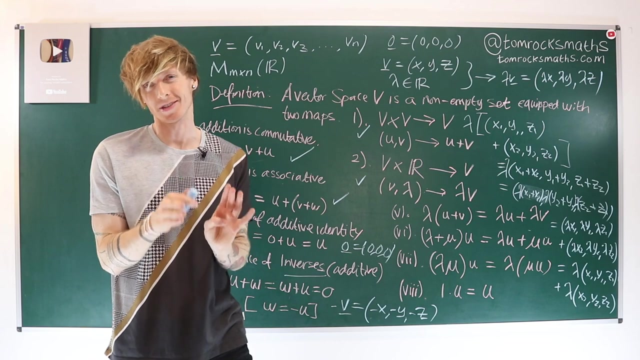 lambda y1 comma lambda z1 plus lambda x2 comma, lambda y2 comma lambda z2.. And that is of course the same as lambda times x1, y1, z1 plus lambda times x2, y2, z2.. Again, this might feel like overkill, but it is important to do this at. 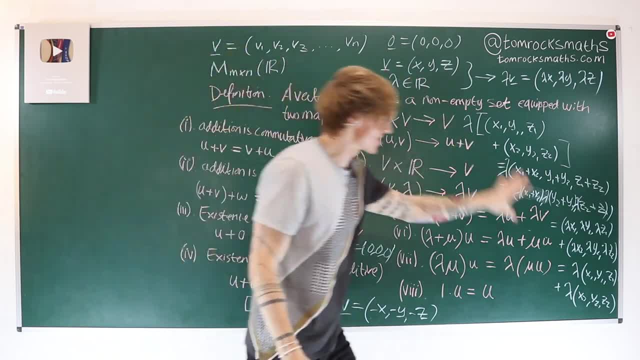 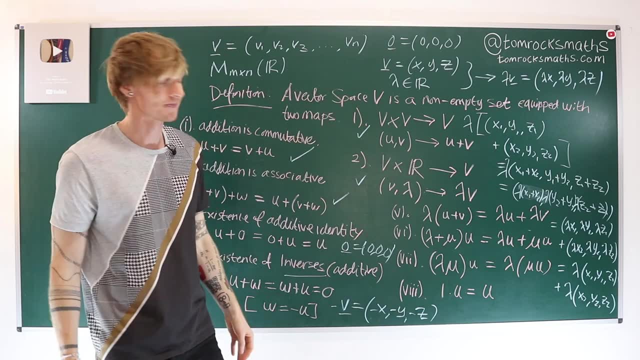 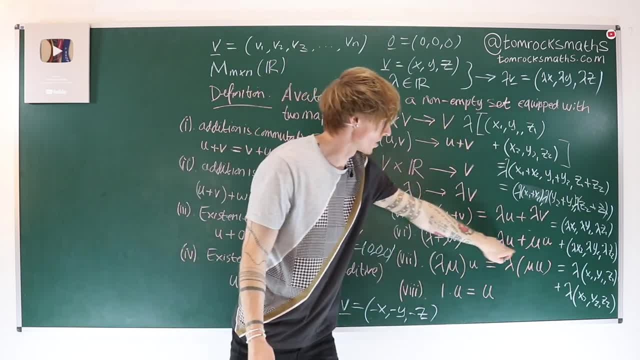 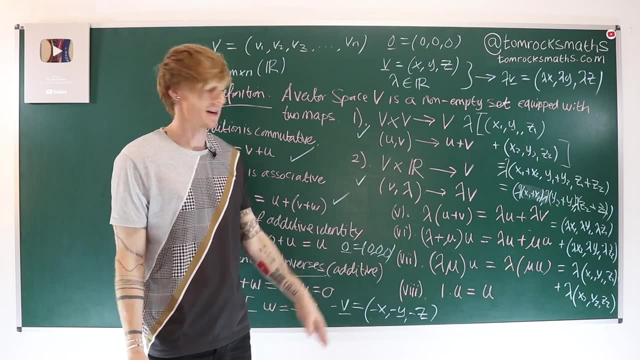 lambda times: x2, y2, z2.. lambda times: x2, y2, z2.. and then I've gone through and we've been able to write it as lambda times, the first one here, plus lambda times the second one. Now, axioms six and seven are very similar. I'm 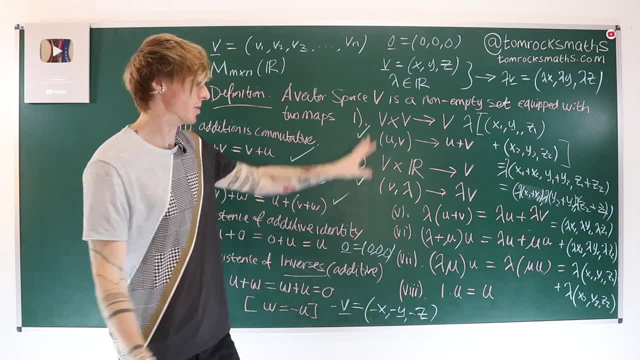 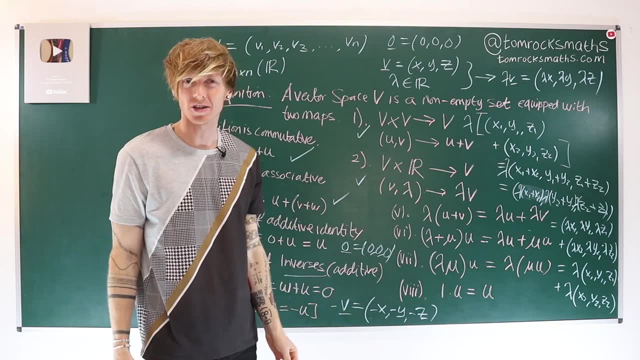 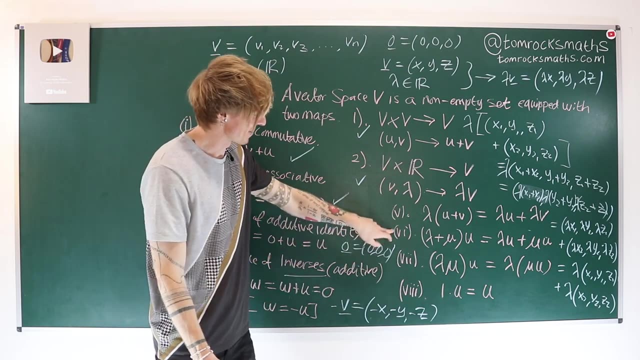 kind of running out of board space and I'm sure you're probably a little bit bored of me writing out all of these very long coordinate addition, sum, scalar, multiplication type operations, So you should check these for yourself. exercise for the audience For six and seven. 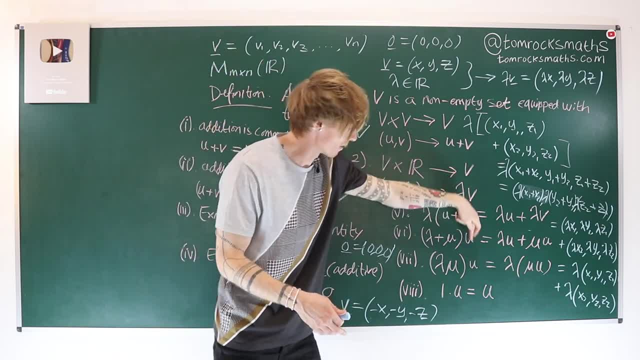 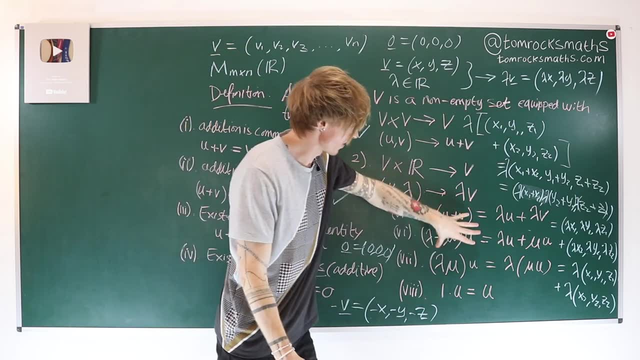 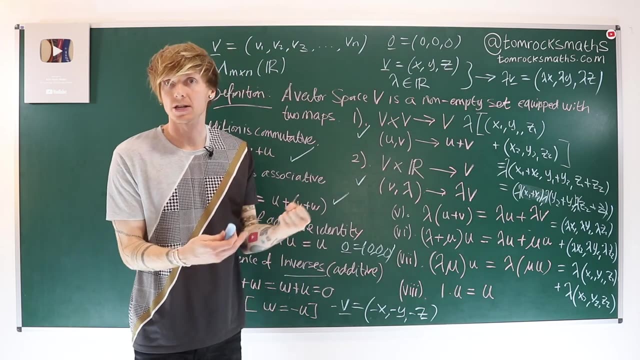 So, again, we just take our general vector u. in both cases, here is going to just be x, y, z or x1,, y1, z1, doesn't really matter- And you just need to convince yourself that the left hand side is the same as the right hand side, following our way that we've defined addition and scalar multiplication. 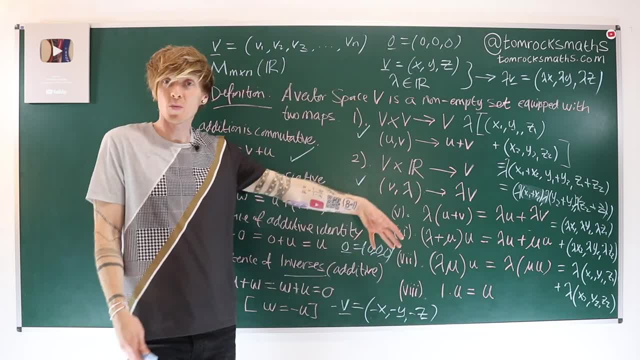 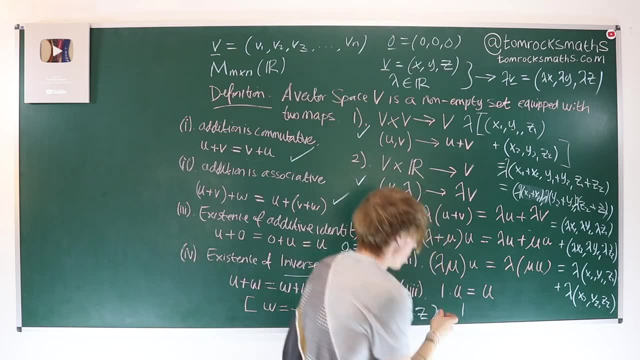 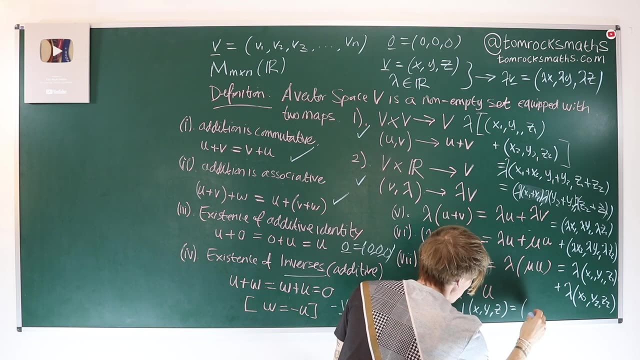 And then, of course, for the final one, we are in the real numbers. So there's not really much to do here except to say: well, our identity is clearly 1.. It's when lambda is 1.. So 1 multiplying x, y, z is definitely going to give me 1 times x, which is x, 1 times y, which is y, and 1 times z, which is z. 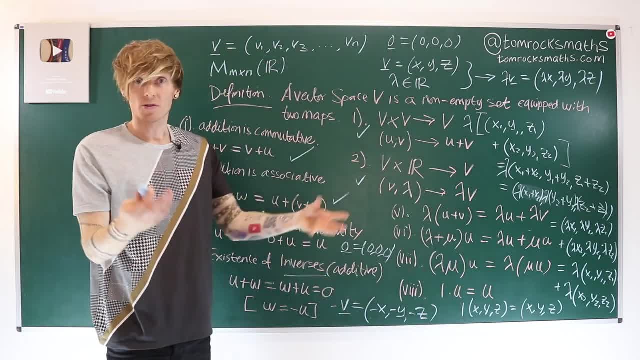 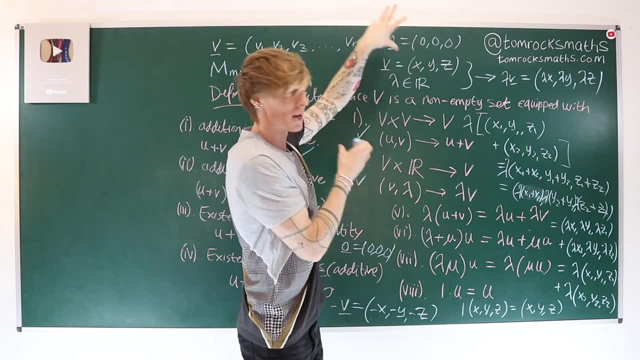 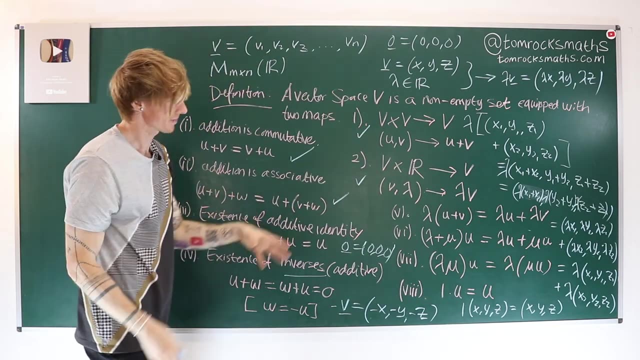 So there's not too much to do for that last one. As you saw, there was a little bit of work in terms of addition and convincing ourselves that the way we're used to adding vectors does indeed fit with the axioms of a vector space. 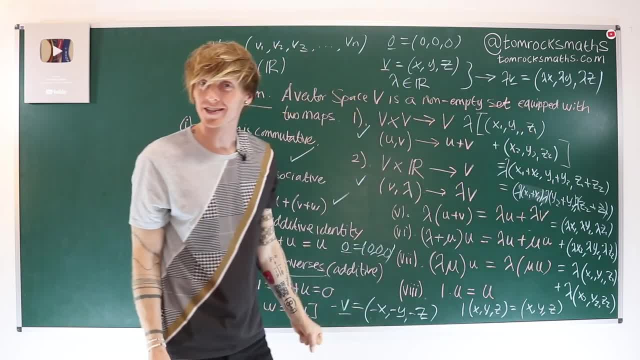 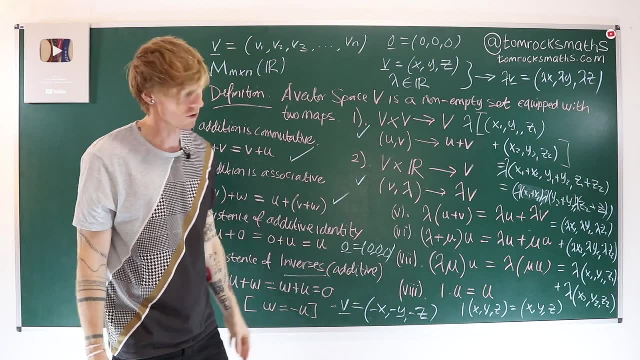 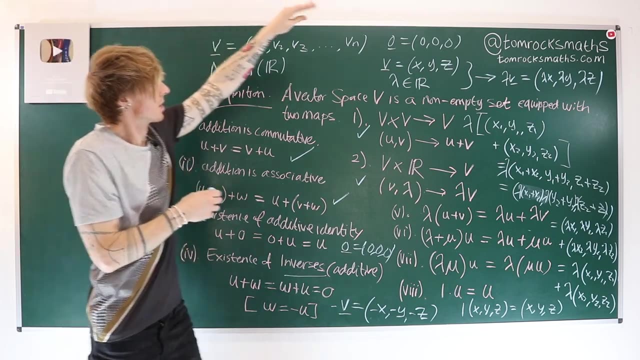 And then we had to do some of these rather mind-numbing expansions, But important nonetheless, to convince ourselves that these rules here- 5 through to 7, also follow And everything also works exactly as it should. So we can conclude that the three vectors 3D coordinates are indeed a vector space. 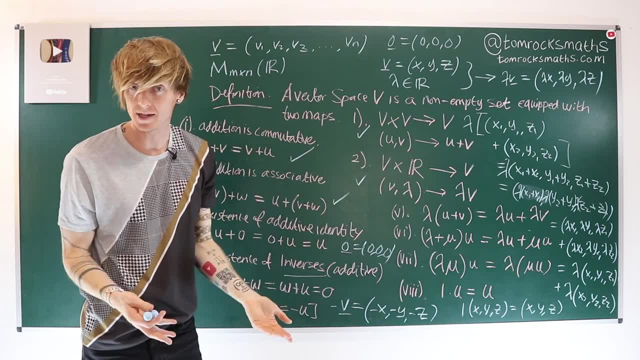 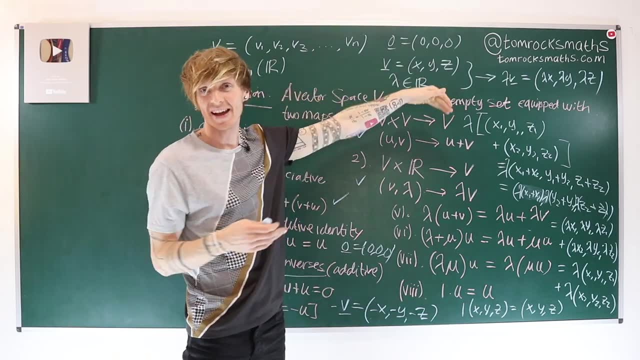 Satisfying all of these axioms and have the two maps with the desired properties. And hopefully you've also realized there was nothing special about me having three vectors here. I just picked three because it's something we're likely to be most familiar with. 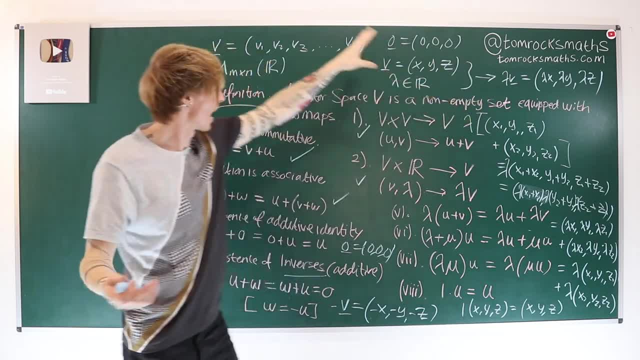 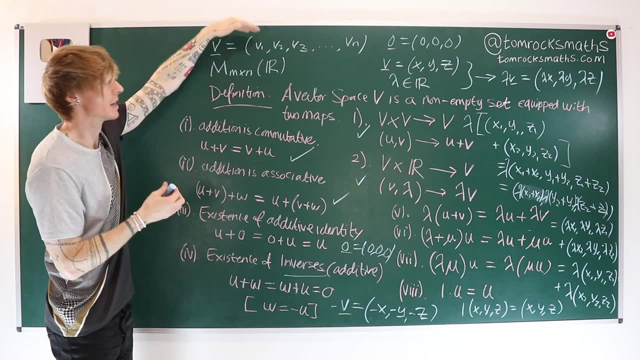 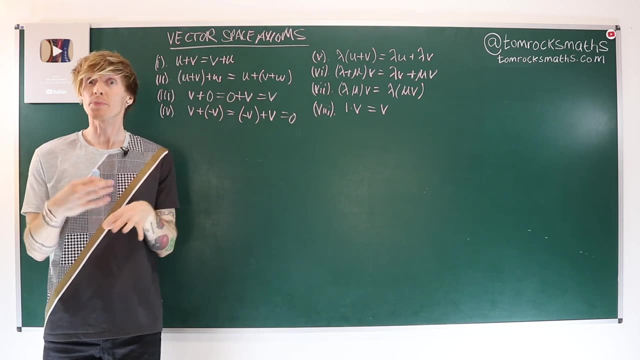 This could, of course, be an n vector of any length, And all of our work would follow in exactly the same way. So we can see that n vectors, as defined here, are going to give us a vector space. Now that we have our vector space axioms, we can actually prove further properties about vector spaces. 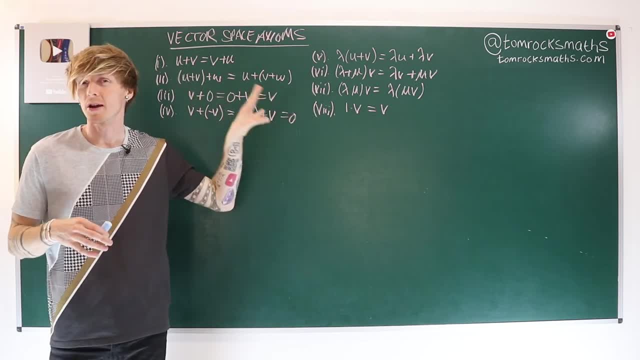 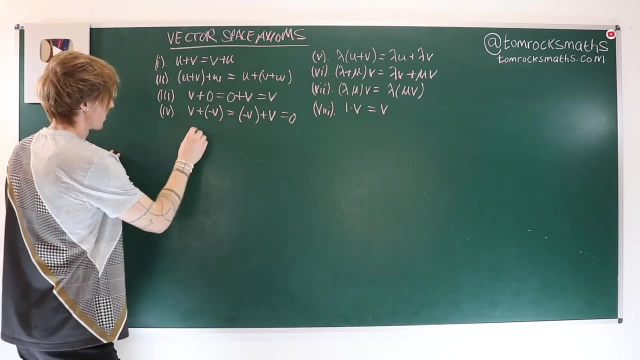 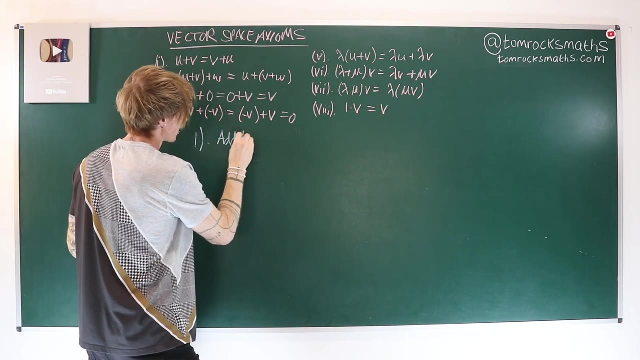 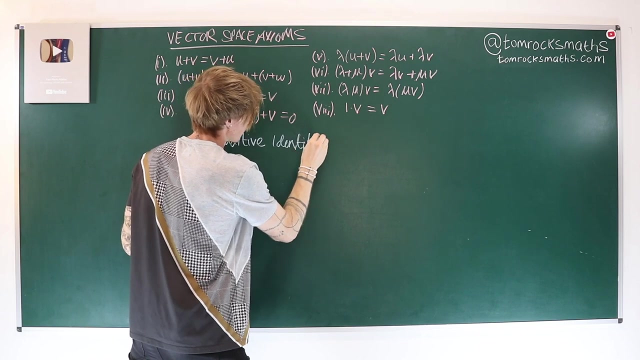 just using the eight rules written on the board. Two of these are particularly important. The first one, which I will label property one, is that the additive identity element. so the thing mentioned in axiom three, the additive identity, is unique, And the second property is very similar. 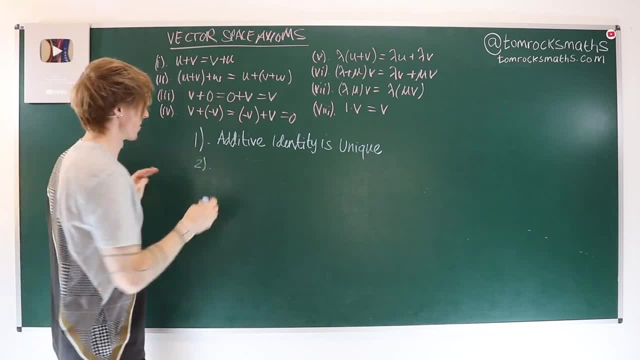 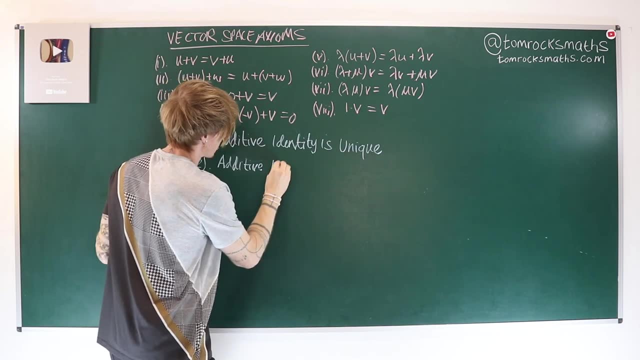 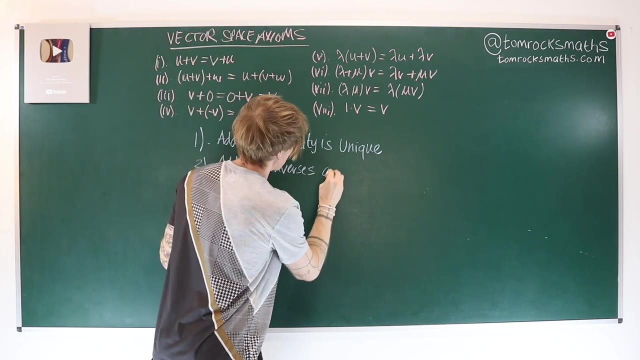 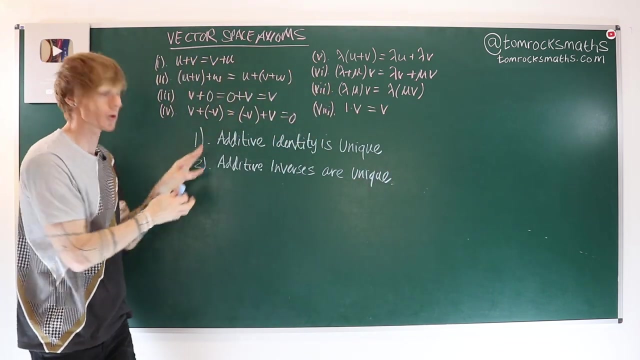 That gives us the uniqueness of inverses, So additive inverses are unique. And, of course, that uniqueness is for each specific element, So additive inverses are also unique. So these are two very important properties to be able to show the uniqueness of these elements mentioned in axioms three and four. 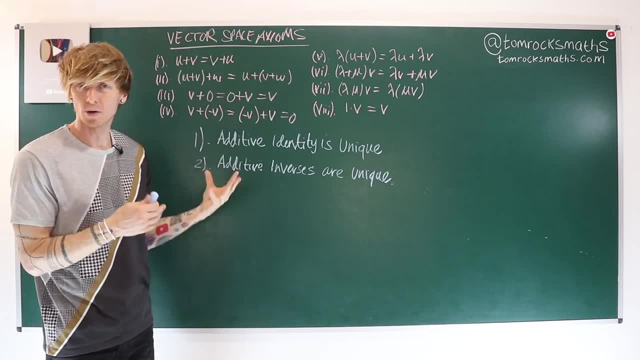 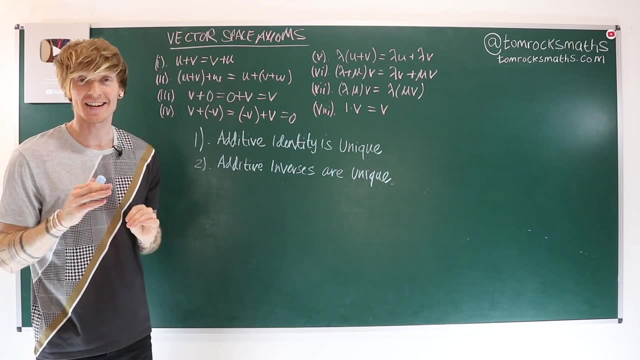 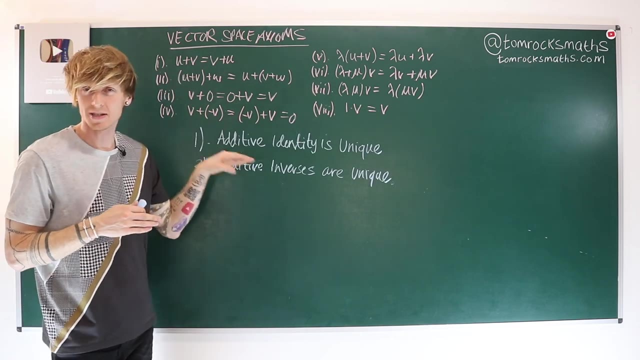 I will go through the first one, because it is important to see how you construct one of these proofs. The second one will be left as an exercise for the viewer, A very useful exercise, I might like to add, And it does follow in much the same way as I'm going to show you how to do the first one. 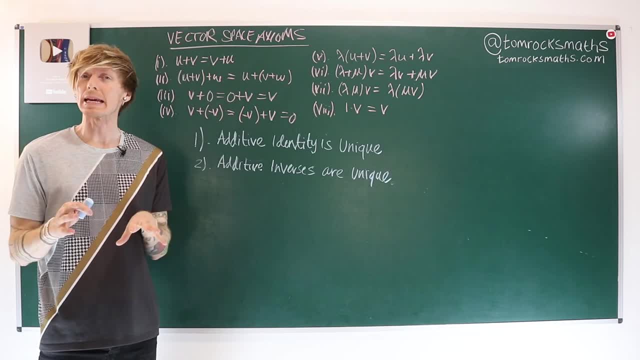 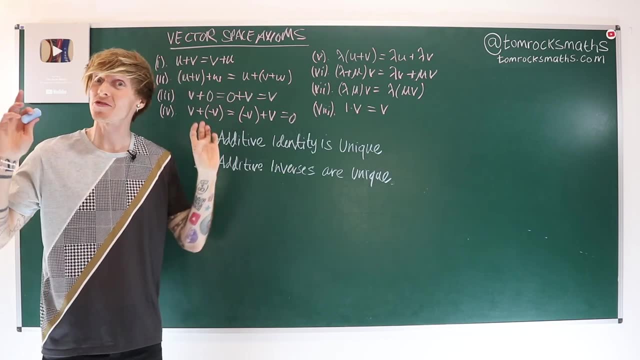 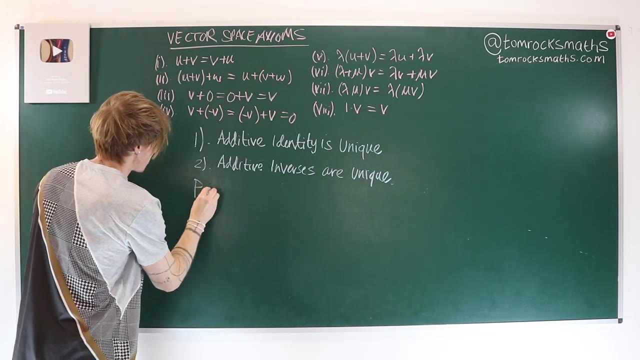 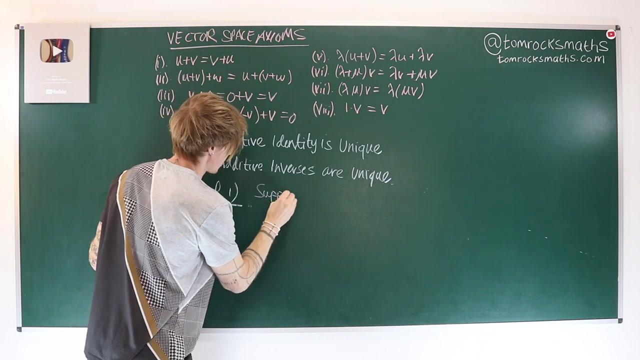 As with most uniqueness proofs, we begin by supposing there are two such identity elements, And our secret goal is to show that they are in fact the same element. So proof of property: one Suppose we have two. So suppose zero and zero prime. 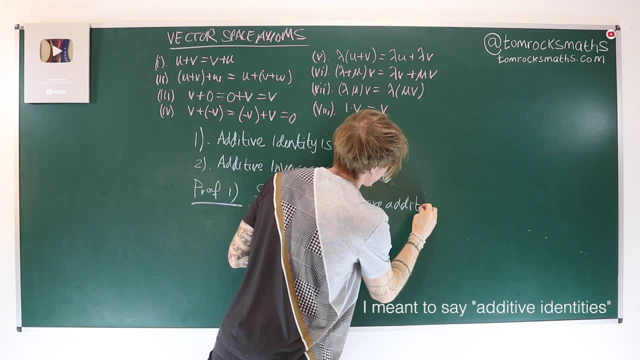 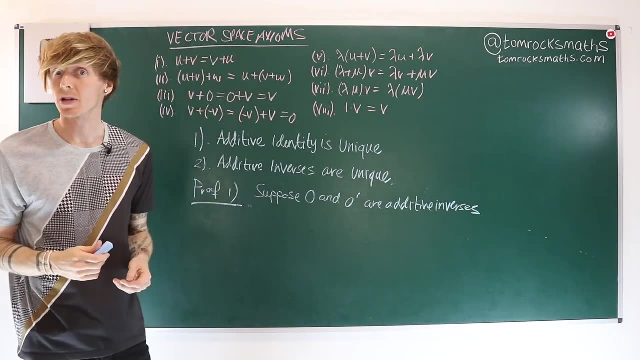 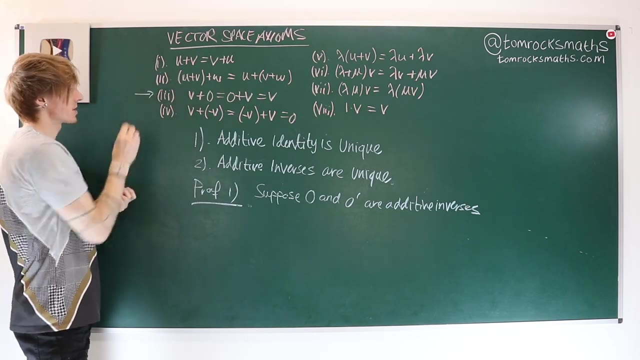 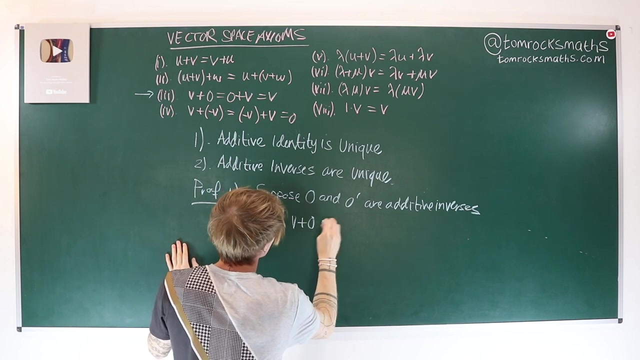 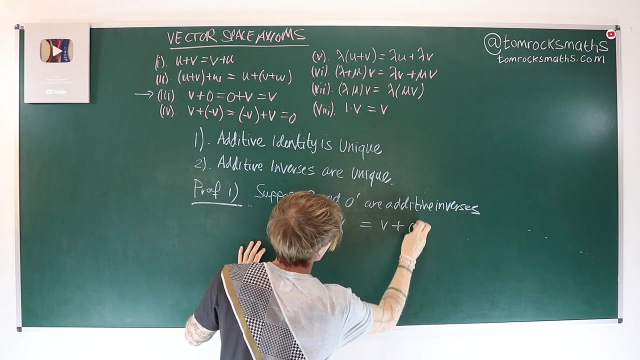 Are additive inverses, Then a sensible starting point is to write out what that means according to our axioms, So according to axiom three. What that means, then, is that V plus zero is equal to V, But also That is the same as V plus zero prime. 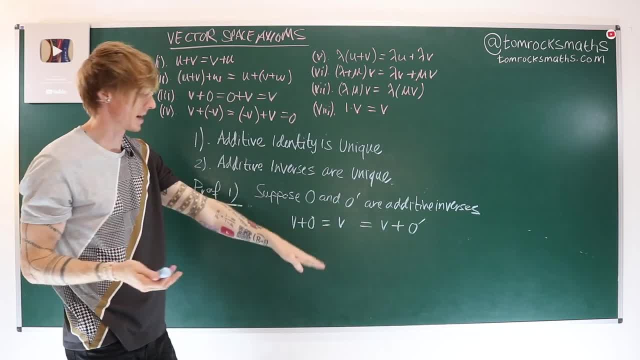 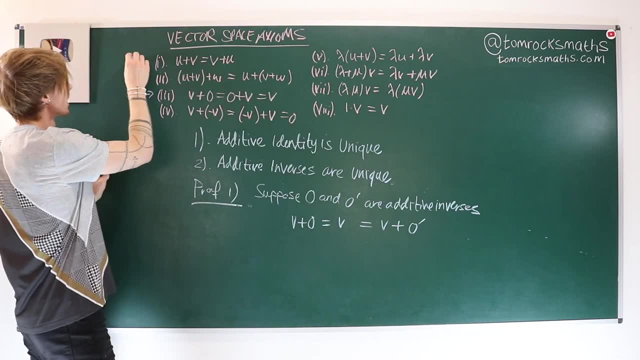 Now We're going to ignore the V in the middle. I just wrote it there because both of these expressions are equal to V, And in fact, what we want to do is now use axiom one, Which says that we can add together things in any order. 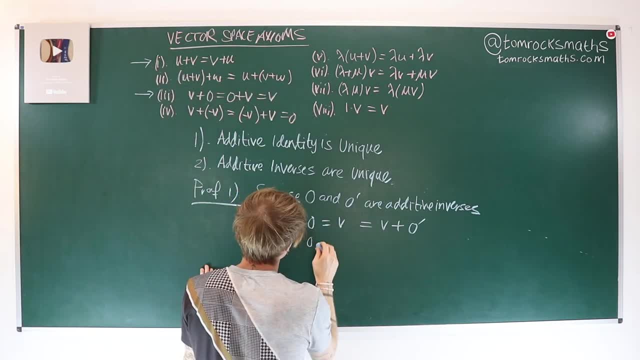 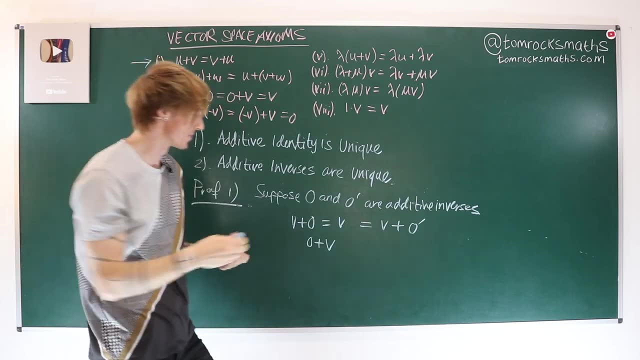 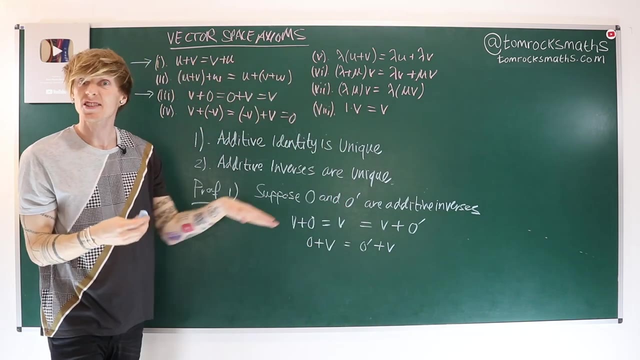 So I can rewrite this now and say: So that means that zero plus V, Just interchanging the order of that addition By commutativity Property one, Is equal to zero prime Plus V By again Interchanging the order there. 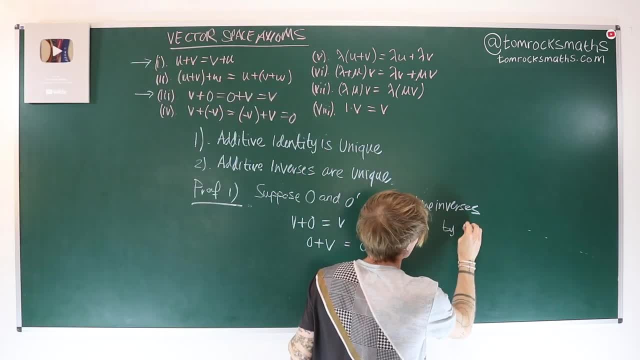 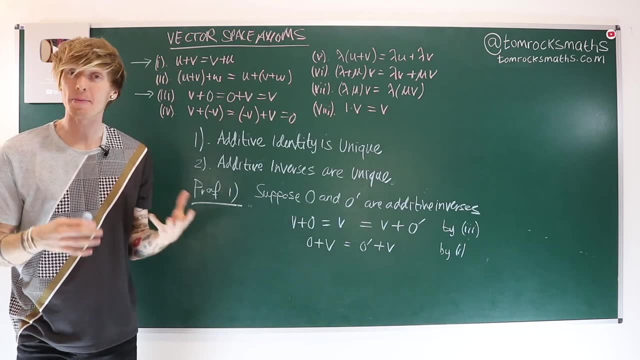 By axiom one. So I should really keep track of what I'm doing. So this one was by number three, And then I interchanged the order By number one. Now the next step in our proof Comes from thinking about our ultimate goal. 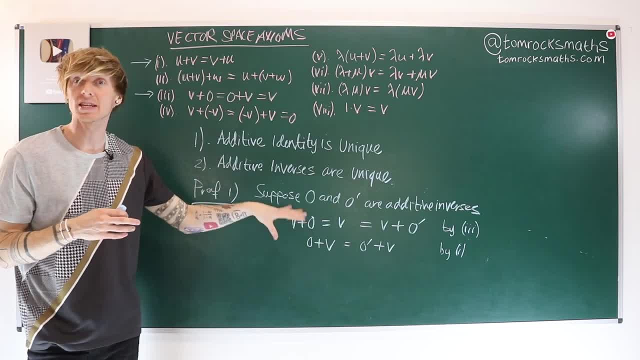 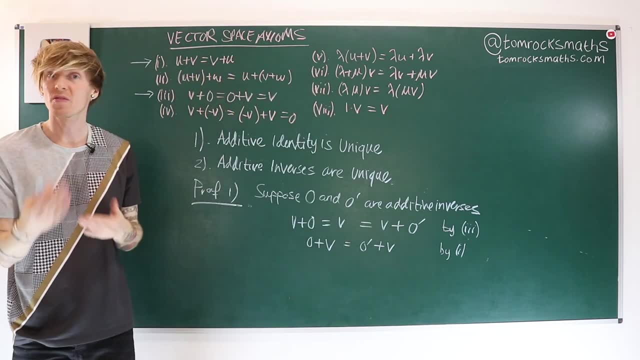 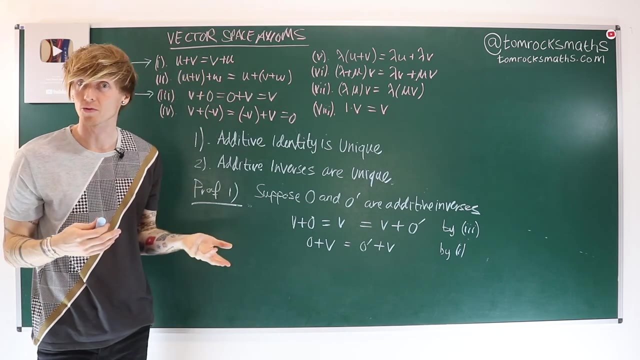 Which here Is to argue that zero is equal To zero prime. So what we want to do Is really cancel this V, But it's not quite as straightforward as just cancelling it, Because we have to use our axioms And we have to use our rules. 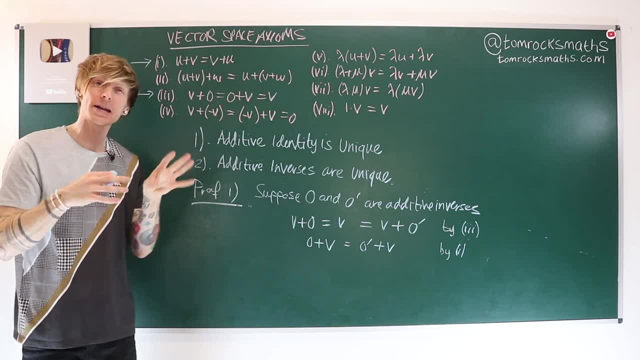 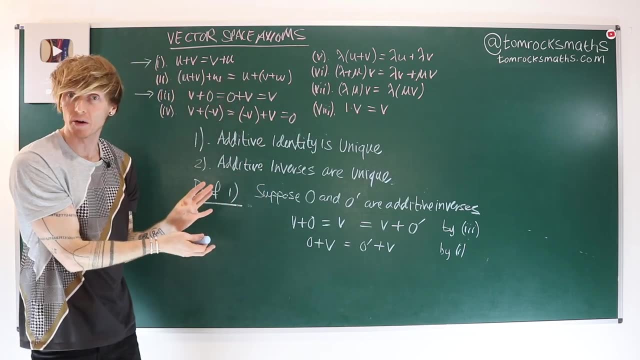 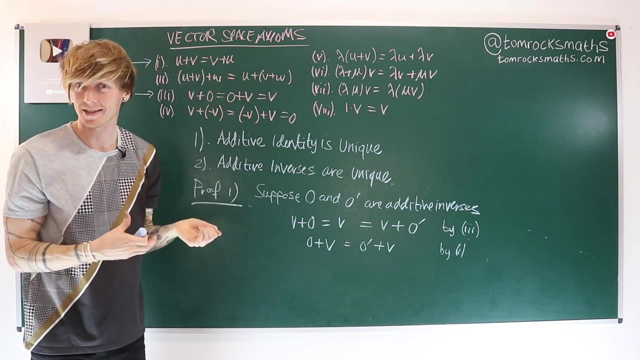 That's how these proofs go. Again, they can be a little bit annoying, But it is important To build up our knowledge And build up the properties Of a mathematical structure Purely based on Those initial assumptions, Those initial rules or axioms. 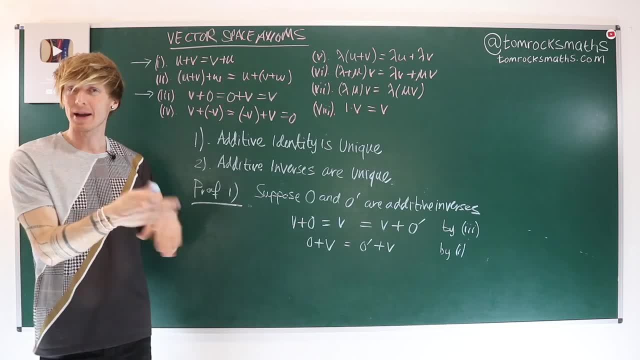 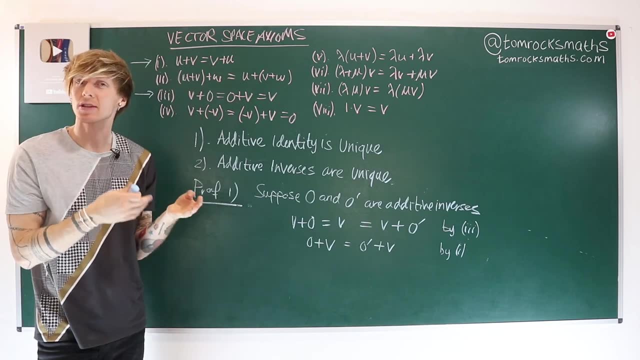 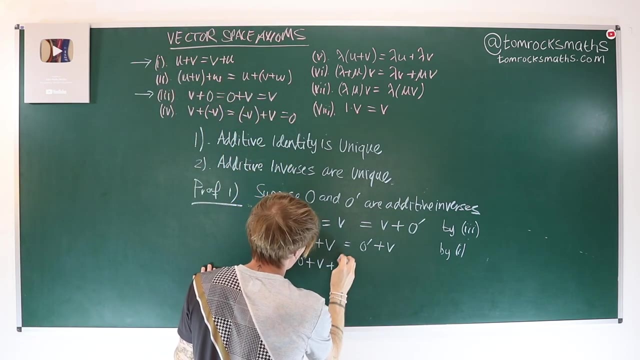 So We kind of want to add a minus V To both sides Because that Possibly, by using axiom four, Is going to allow us to cancel The V. So if we do that We can say Not plus V, plus minus V. 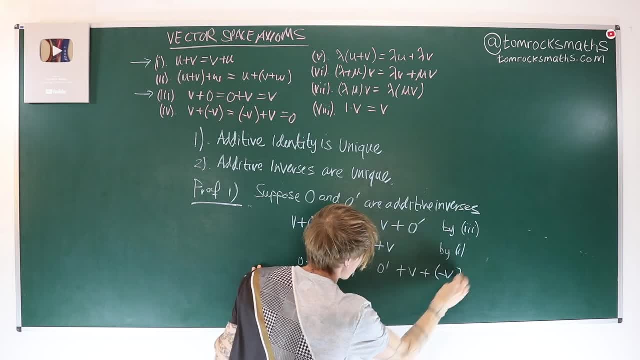 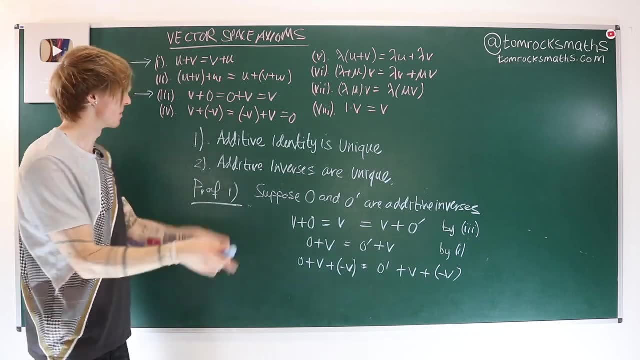 Is therefore equal to zero: prime Plus V, Plus minus V, And now we have three terms on both sides. So what we actually need to do here Before we can use four, So we want to use four, But before we do that, 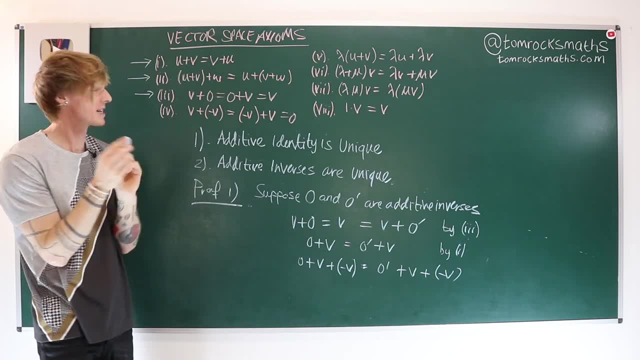 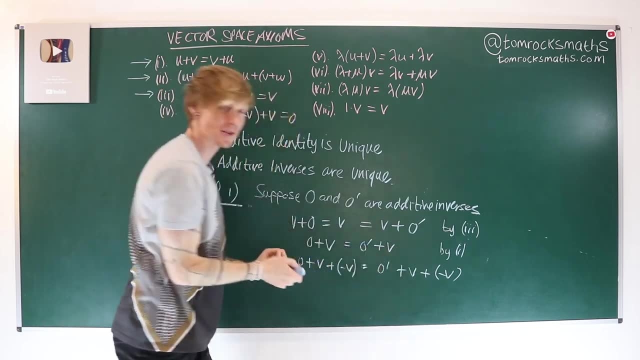 We actually need to use two. We need associativity, We need to make sure that what we're allowed to do here Is actually add The second and third terms together On both sides first, And then be okay, So we can do that. 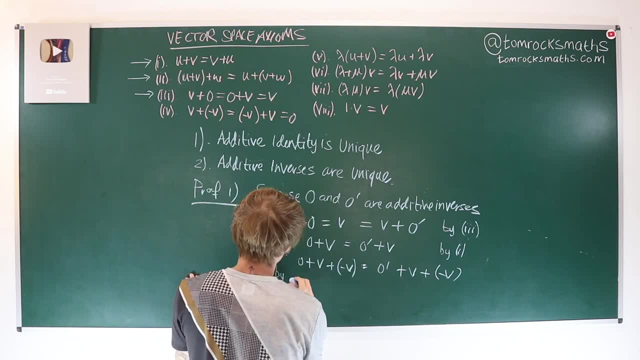 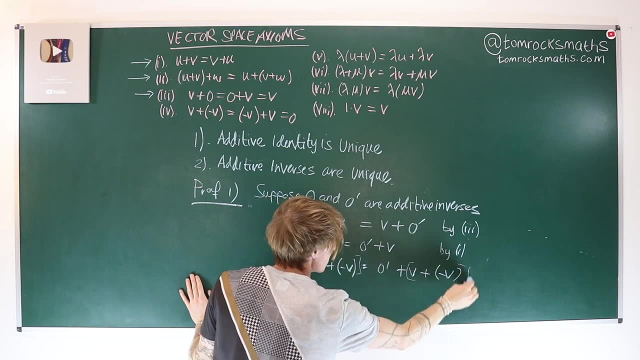 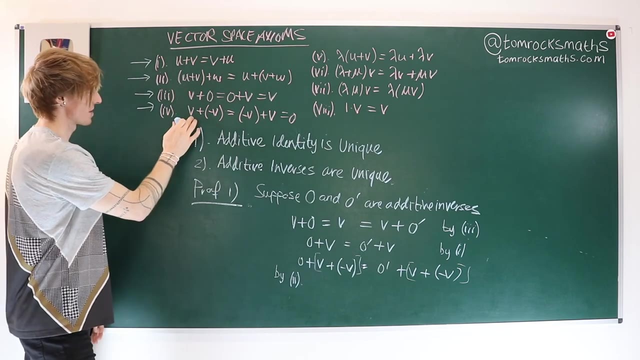 And say: by Associativity Plus two, We can then say That's the same as adding those two And those two. And now, Finally, We can use axiom four And say, well, V plus negative V, That gives us our identity element zero.